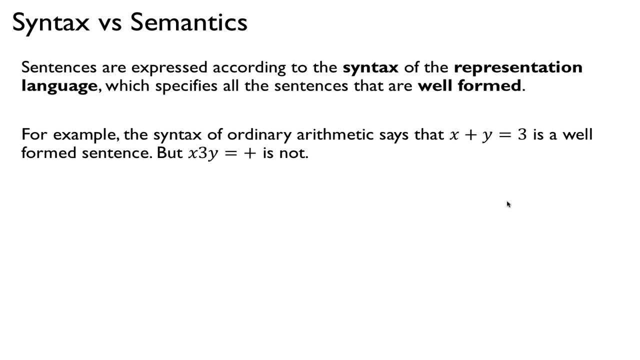 That's a well-formed sentence. That's a well-defined, well-formed sentence And it follows and satisfies the syntax of basic math. But something like x, 3, y equal plus is not a well-formed sentence. that follows the syntax of basic math. 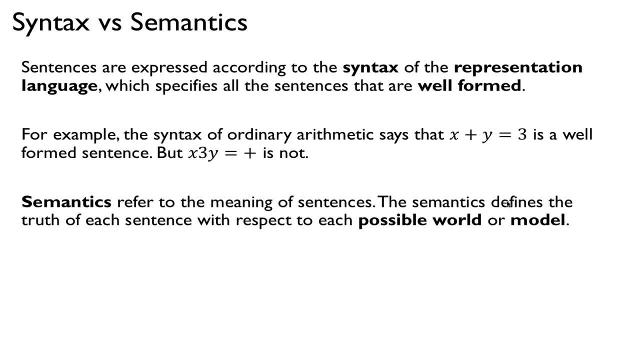 So syntax is basically the form of the language, And then semantics refers to the meaning of the sentences. The semantics defines the truth of each sentence with respect to each possible word or model. So a model is this. Let's do an example here. 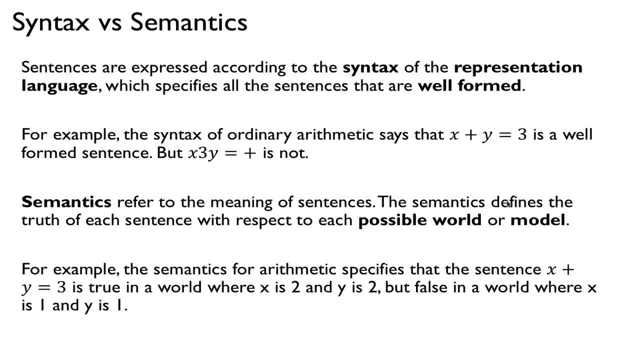 Semantics of again, basic math says that when you have a sentence like x plus y is 3,, then that sentence is true in a word or in a model where x is 2 and y is 2.. Sorry, x plus y is 4, rather. 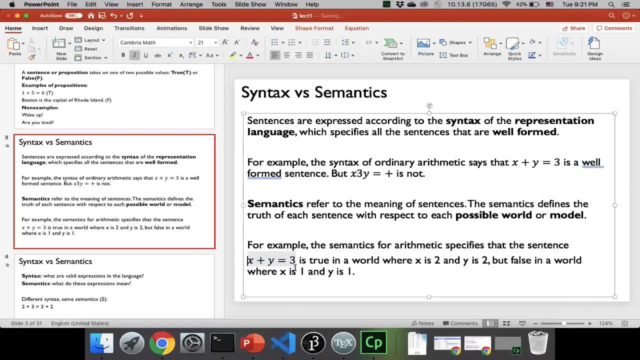 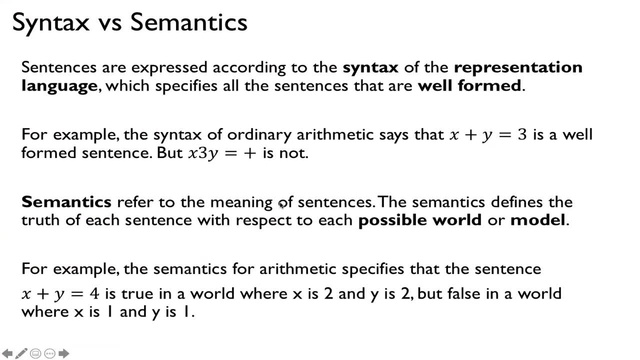 Sorry about that. And so if you have an equation like x plus y is 4, then in a word or in a model where x is 2 and y is 2, then this statement is true, But in a different word or a different model. 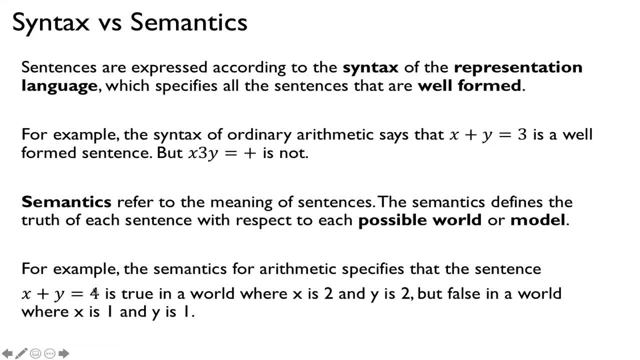 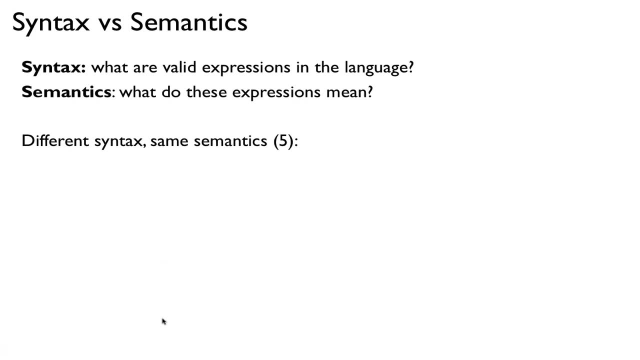 where x is 1 and y is 1, then this equation is not true And so these sentences have meanings when we assign values to the sentence. So again, syntax is basically the valid expression in the language. Semantics is basically the meaning of those sentences. 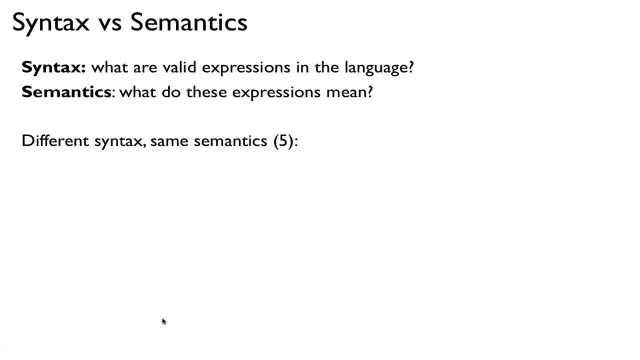 So, for example, here's an expression that has different syntax but same semantics: 2 plus 3 is equal to 3 plus 2.. So 2 plus 3 is a different syntax than 3 plus 2, but they both have the same semantics. 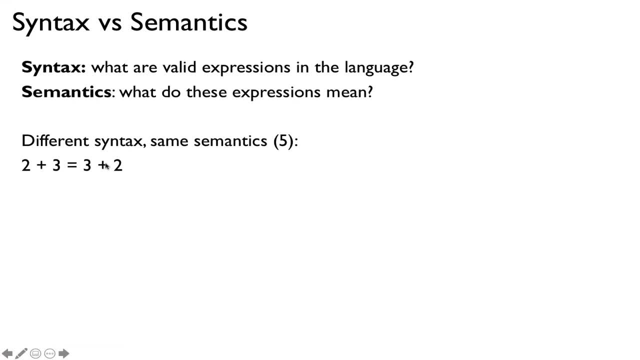 They're both equal to 5.. So even though the syntax is different, the meaning is the same. But here's an example where the syntax is the same but the semantics is different. So if you've done some programming and if you haven't, 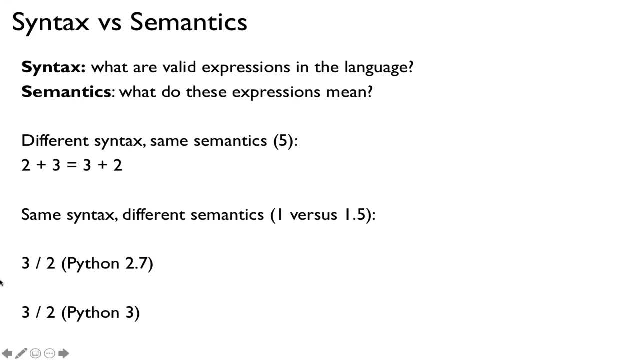 in Python 2.7,. this is the old Python. this is the programming language. 3 divided by 2 uses something called floor division. 3 divided by 2 is throw away the decimal, So that 3 divided by 2 is actually 1.. 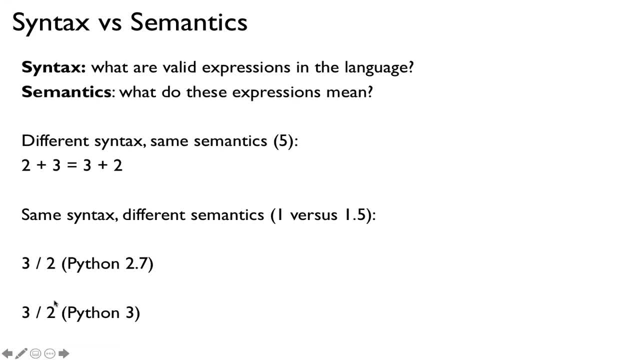 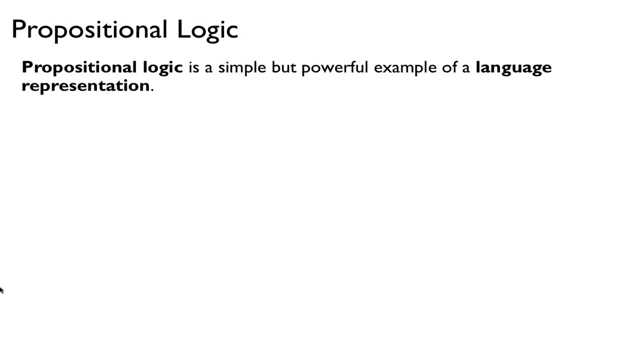 And then in the new Python, Python 3,, 3 divided by 2 is true division. So 3 divided by 2 is 1.5.. So even though the syntax here is the same, the semantics is different. It depends on which Python version you're using. 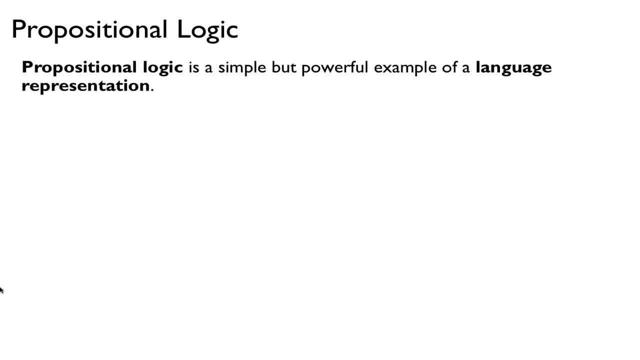 Okay, so we've been talking about a language representation, And so let's give you an example of this. So propositional logic is a very simple but very powerful example of a language representation. So let's talk about the syntax of this logic. 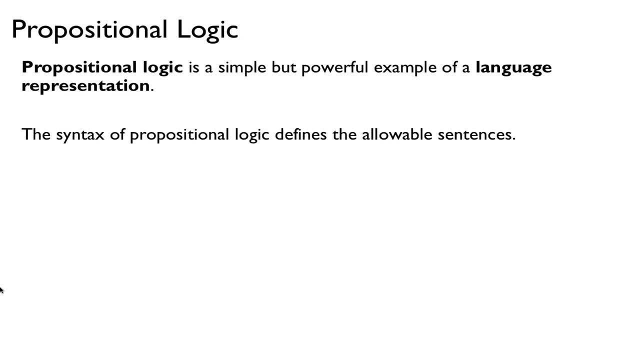 It defines all the sentences that are allowable or the sentences that are valid according to the syntax. Atomic sentences, basically, are very simple. They consist of only a single proposition symbol. Each symbol stands for a proposition that can be either true or false. So, for example, let P be a proposition symbol. 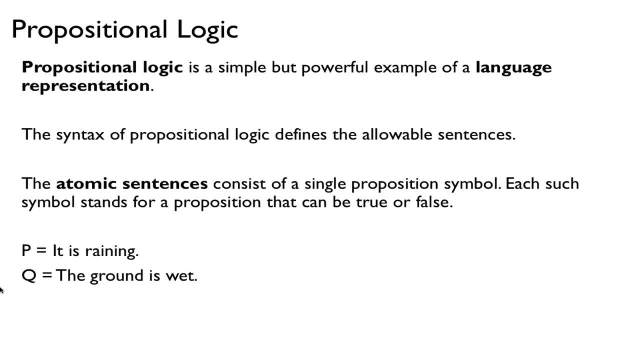 It represents it is raining. That could either be true or false. Q is another single proposition symbol. It represents the ground is wet, And so these are called atomic sentences. It's just a very basic sentence that we're going to use to build up. 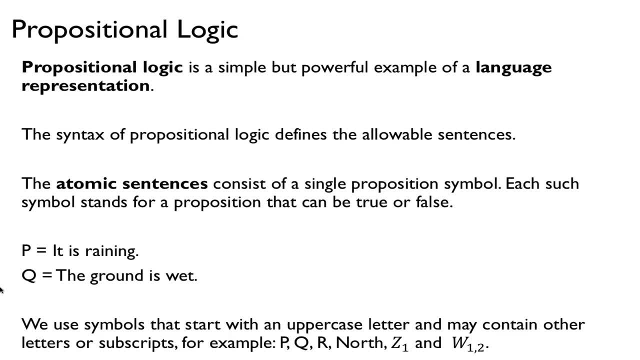 more complex sentences, So these are called atomic sentences And, of course, when we have a symbol- a symbol could be- We usually use an uppercase letter. We also can contain letters or subscripts: P, Q, R, North, Z1, W12.. 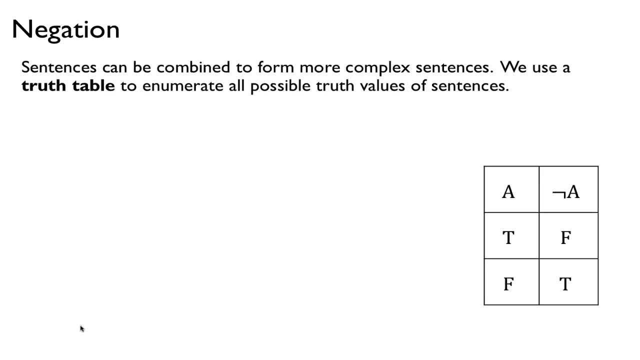 We can use any of those as our symbols. Okay, when we have a bunch of sentences, we want to combine them to form more complex sentences. So, And then The way we're going to explain this is that we're going to go to a bunch of operations. 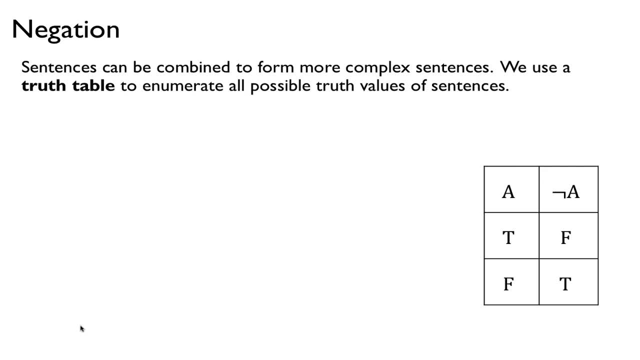 and explain it using something called a truth table, which is a list of all possible truth values of these sentences. One of the most basic operations is the negation operation. It's a unary operation, That means that it acts on one operand. This symbol is this symbol right here? 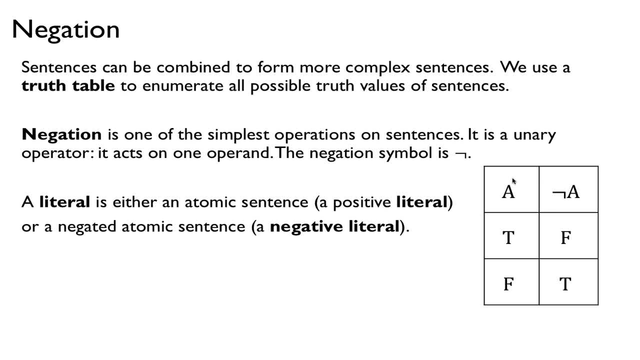 And So what is the negation? Well, if you have one operand, A, A could either be true or false. so in two cases The negation of A will just flip it: True becomes false, False becomes true. So that's it. 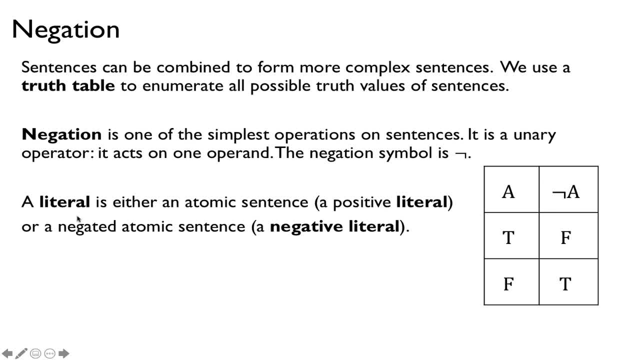 So we say that a literal is another word for an atomic sentence, And so we distinguish between a positive literal right A is a positive literal, which is an atomic sentence, either true or false, And it's just a proposition symbol, in particular. 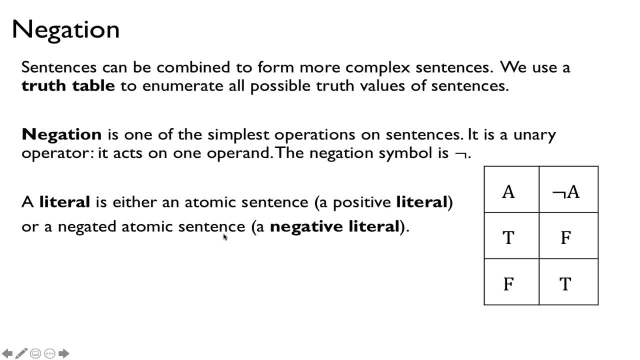 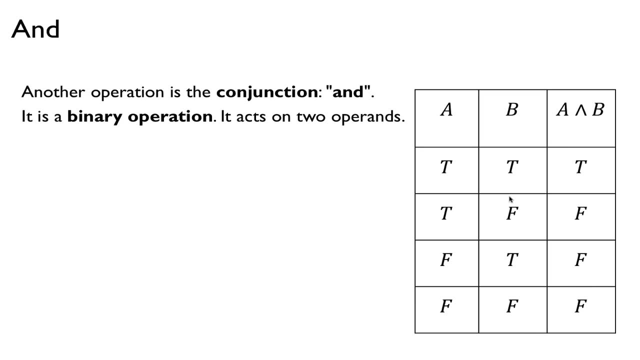 And a negated atomic sentence. we call that negative. literal is the negation of A, So these are called literals. Another operation that's important is called conjunction or the N operator. So this is a binary operation. It takes two operands. 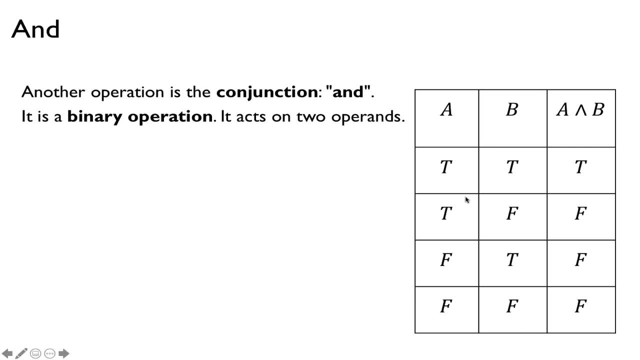 So the way we'll see is that we have two operands, A and B. These are the four cases that they take values on. A and B have either true or false values, So A and B is true exactly when both A and B is true. 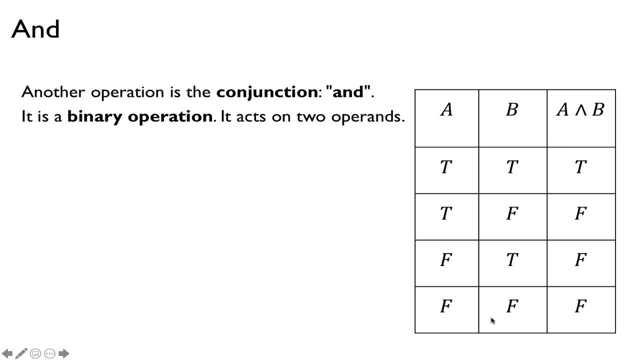 Otherwise A and B has a value of false. So this is called the conjunction of sentences A and B And it's denoted by this symbol. It's kind of like an inverted V, inverted U And, I guess, inverted V. 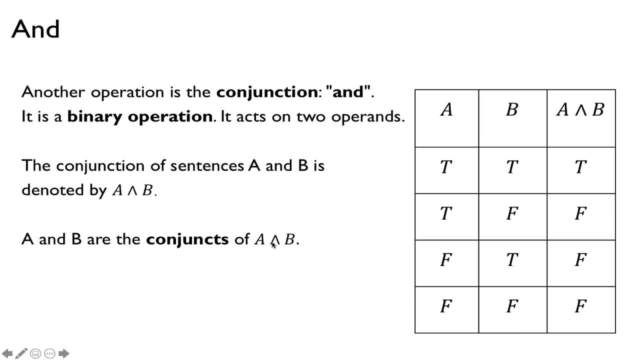 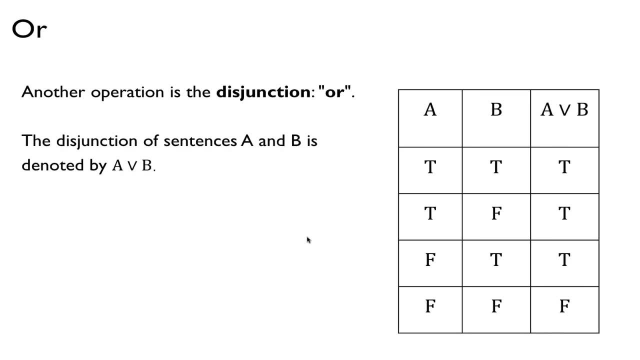 A and B are called the conjuncts of this conjunction. So, And then there's another one. It's the disjunction or the OR. The disjunction of sentences A and B is denoted by A and VB, So this is the symbol for disjunction. 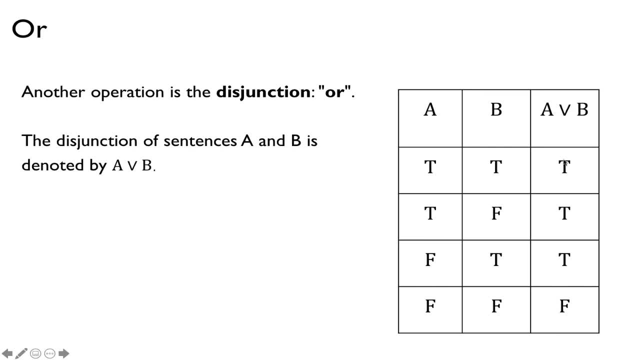 And And. so here's the true table: A or B. A or B is true if at least one of A or B is true. So if both of them are true, or at least this one, A, is true, this one, B, is true. 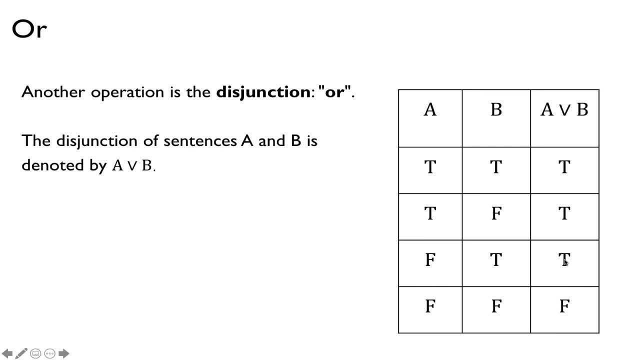 then in any of these cases A or B is true. But if both of them are false, then A or B is false. So A and B are. These propositions are called the disjuncts of A or B, And so this is actually the inclusive OR. 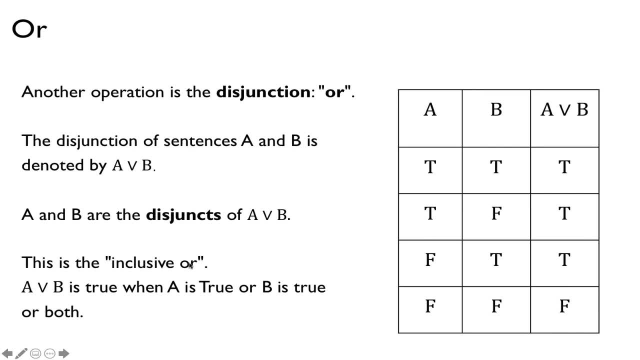 And so there's In math and also computer science. there's also the exclusive OR, And the inclusive OR is actually not. Sometimes in English we actually use the exclusive OR, So the inclusive OR just means that we include both, With the case where both A and B is true. 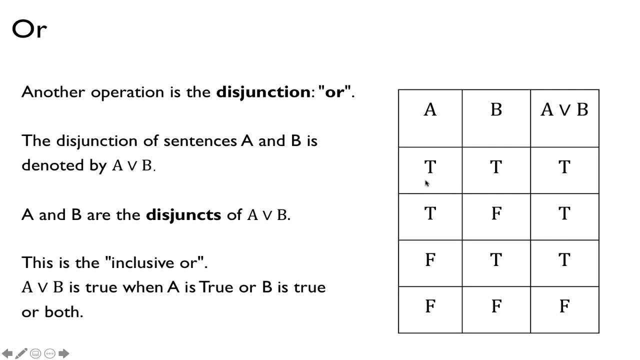 we let that be true. So maybe I'll give you an example. If I go to, say, a restaurant and say Olive Garden and they ask me if I want soup or salad- Again, soup or salad- They probably- You probably- can't say both. 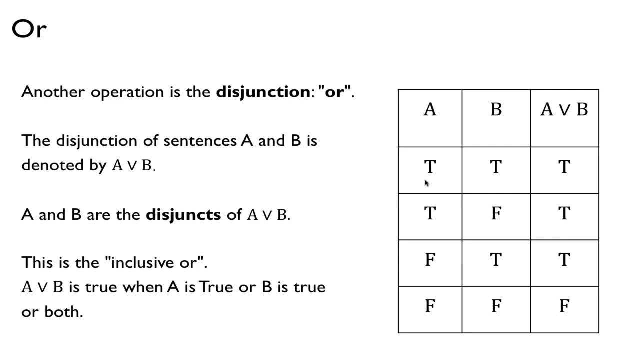 because when they say that they actually mean the exclusive OR, Do I want soup or salad, but not both? So that would be kind of the traditional use of OR is the exclusive OR, But here, in this case, we want to use OR as the inclusive OR. 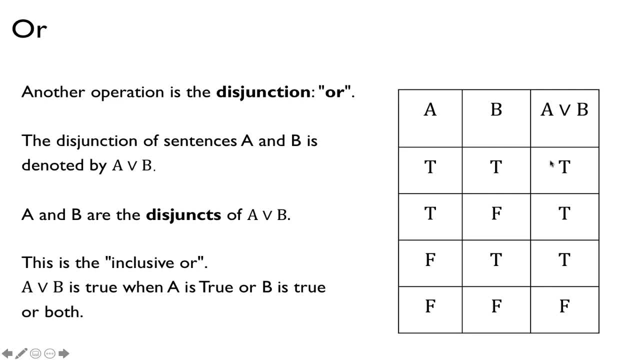 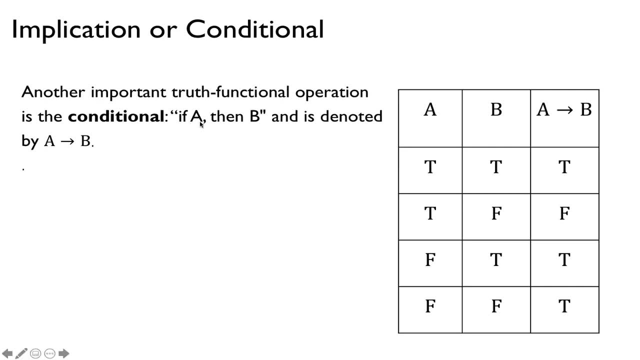 If both A and B is true, we allow that to be true, Implication or conditional. So this is the familiar. if A, then B. So, as you know, by this arrow, this is the conditional, or the implication, Or the implication operation. 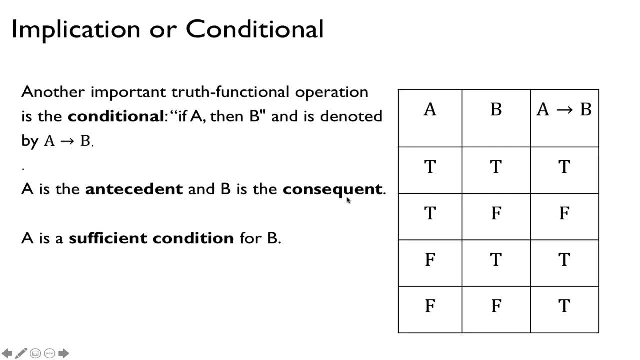 So A is the antecedent and B is the consequent. In other words, if you've done math, you've seen this before- where A is the sufficient condition for B, and then we say that B is the necessary condition for A. 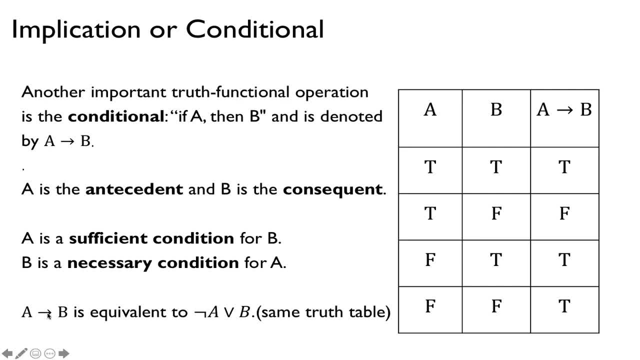 Something that we see later is that it turns out that this conditional is related to the two other operations that we've seen, which is that A condition B is equivalent to not A or B. In other words, have the same truth table In one of the homework for this week. 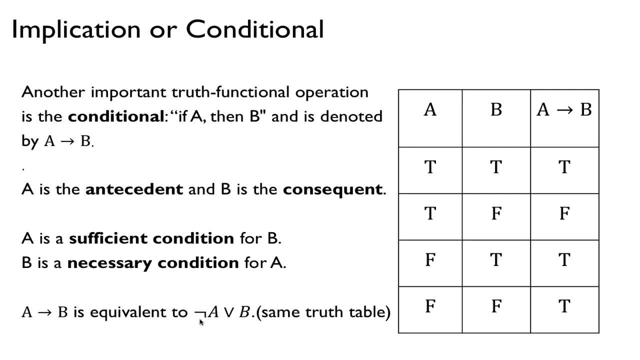 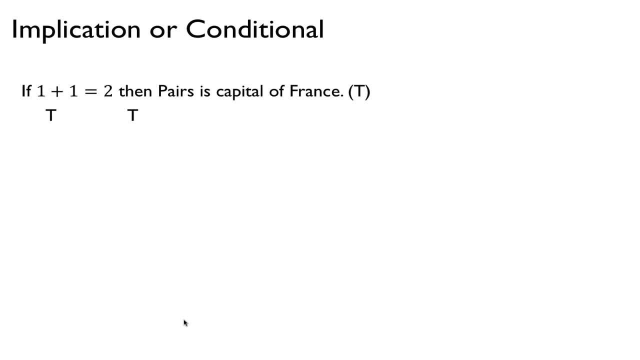 you get to kind of show that This is kind of confusing. so I want to use a more example of this implication operation. So let's look at this: If 1 plus 1 is 2, then let's just say Paris is the capital of France. 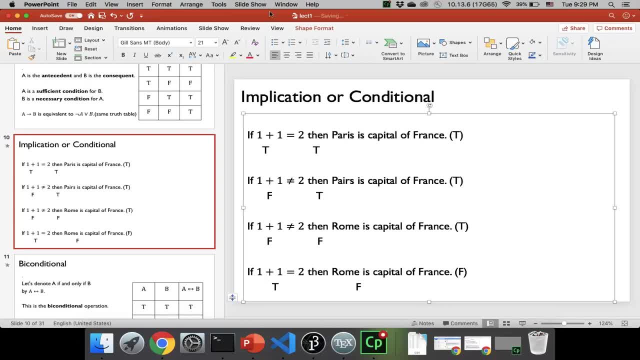 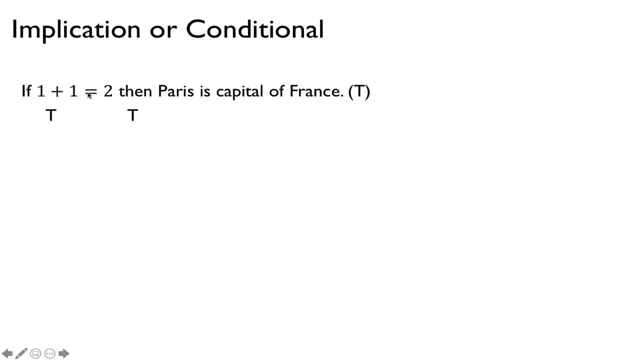 Okay, so why does this have the value of? Well, this is kind of a simple example, but let's do that again. So notice: this part of the conditional is true: 1 plus 1 is 2.. And then Paris is the capital of France. 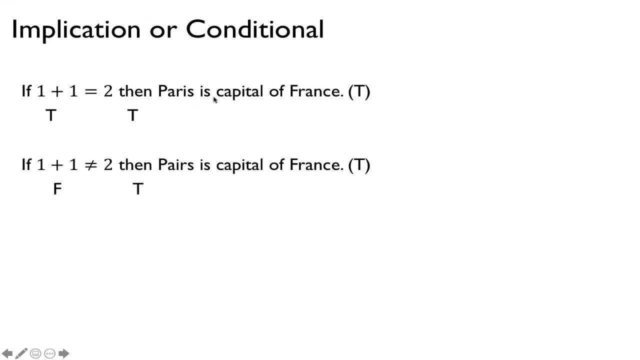 So if this is true- and this is true- then the whole thing is true. Now this is where it gets a little confusing. If this is false: 1 plus 1 not equal to 2, that's false and this is true. 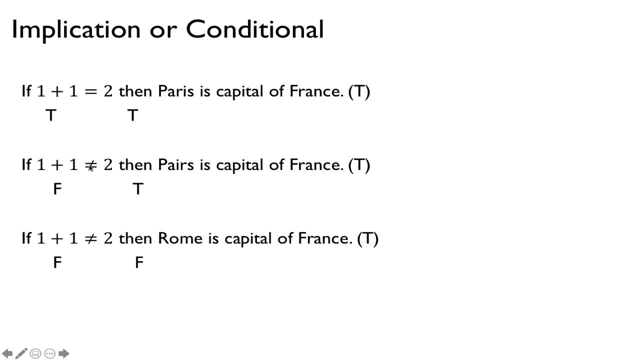 but we're going to let the whole thing be true. So, even though the conditional, this antecedent- is false, but we let this whole thing be true. So why is that? And the idea here is that Let's go back to this. 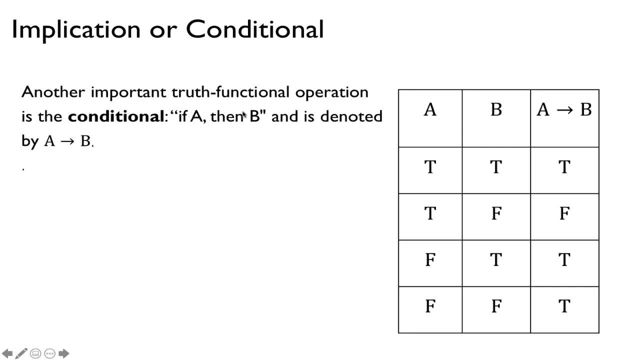 So if A, then B, If A is true, then B is also true. But if A is false, then really we're going to say that this sentence is true. This is vacuously true, because if A is false, then this doesn't apply. 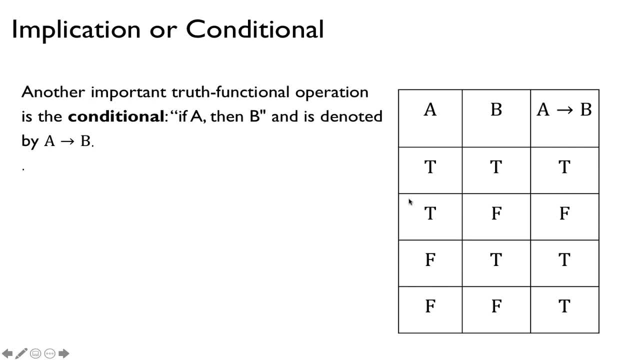 and so we're going to say that this statement will be true. So again, if A is false, then regardless of what B is, we're going to consider this conditional to be true. So this is kind of confusing, but that's how we're going to disagree on that. 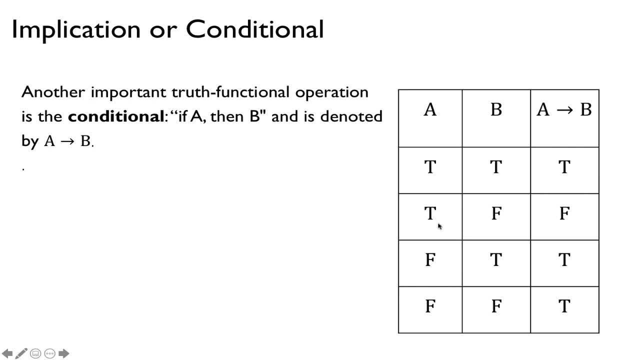 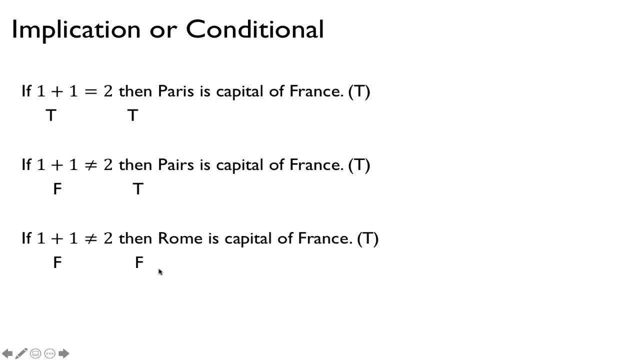 And then certainly, if A is true but B is false, then definitely that's going to be false, And so let's do some more examples here. So if this is false, then it doesn't matter what this is. Is it true or false? 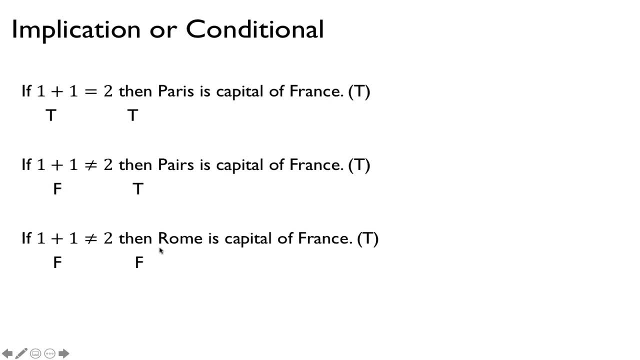 So if A is false, then it doesn't matter what B is, The statement will still be true. But this is the case where the statement will be false. If A is true but B is false, then definitely this conditional is false. 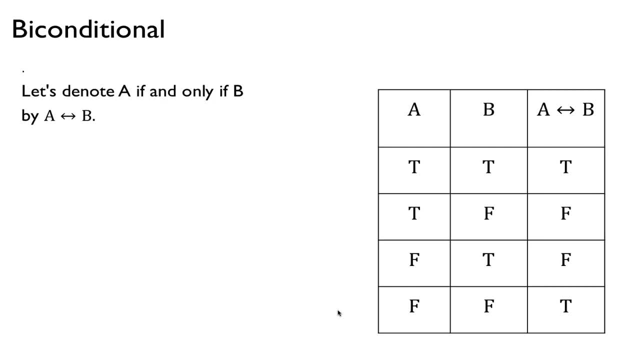 Biconditional. Let's denote A. Let's denote this by using a double arrow. So this is the biconditional operation And basically this: A biconditional B is true when, and only when, A and B have the same truth value. 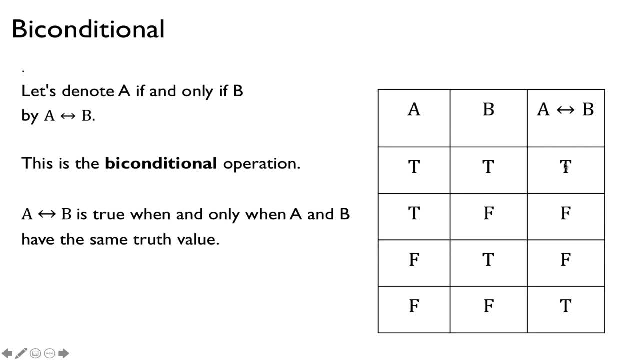 So in other words, if I notice here, this is true because they have the same value, And then it's true again because they have the same false value. But if they have different value, then the biconditional is false. So biconditional is to know that they have to be the same to be true. 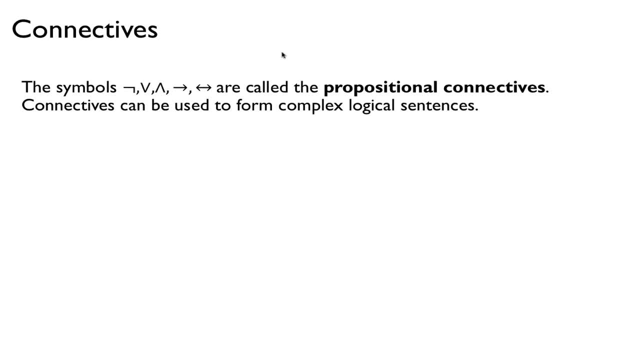 Okay, so these are connectives. We have seen so far five connectives: The negation, the before the and the implication and the biconditional. So these are called propositional connectives And they're used to connect sentences and form more complex sentences. 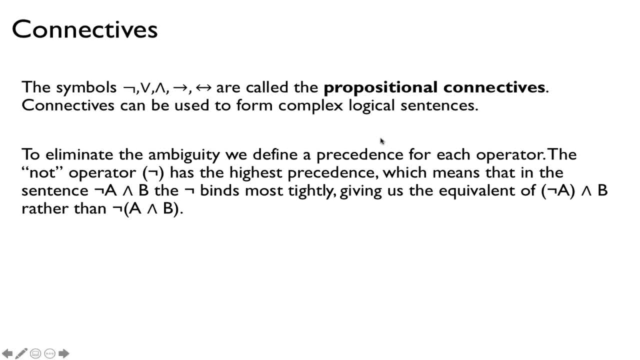 So one thing to kind of be clear is that we're going to define a precedence or an order of operation. because we have all these different operations, We're going to put that the NOT operator had the highest precedence, In other words, without parentheses. 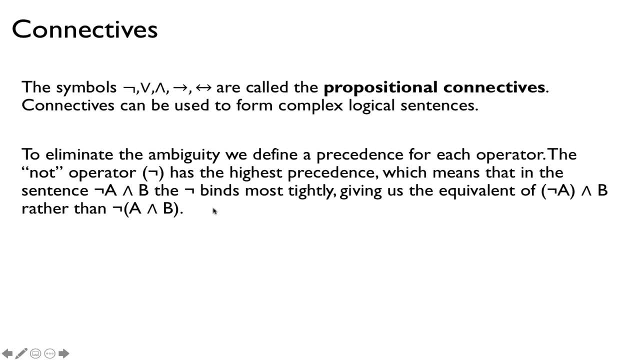 the NOT is going to be done first. So, for example, we're going to do NOT A AND B, The NOT A is going to bind to A. The NOT is going to bind to A first rather than binding to the AND operation. So we're going to do NOT before the AND. 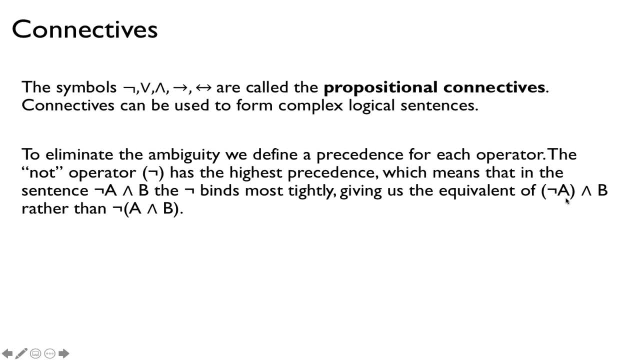 So this means NOT A and B, So that has the high precedence And then I guess, the other. I guess I didn't make clear here, but the We're going to put the. The next operation is we're going to do AND before OR. 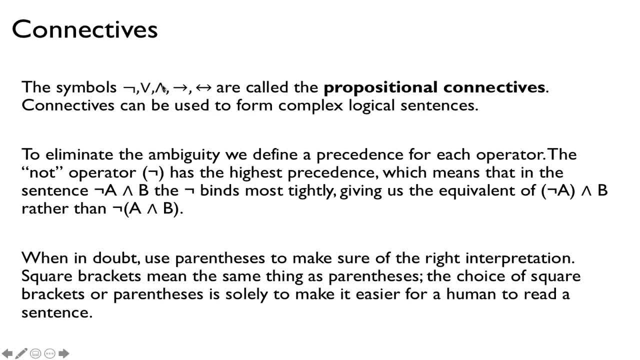 And then: So that's going to be something that, Even if you've done Java or Python, yeah, so in programming the AND operation is done before the OR operation, for example. Okay, Let's see. And then parentheses: we can use that to kind of make things clearer. 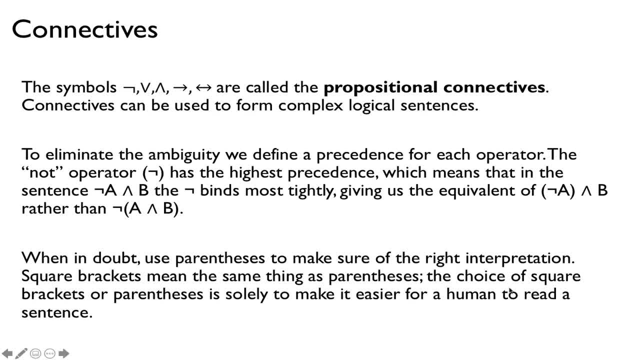 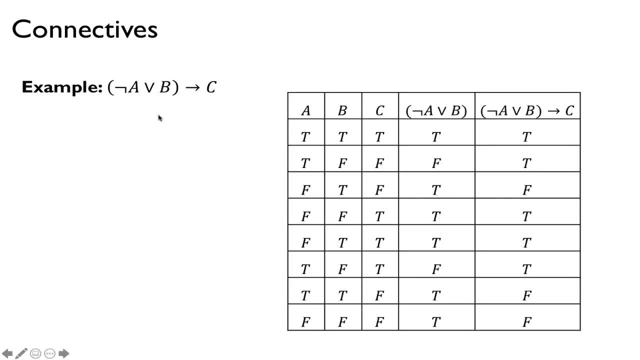 You can use a regular Regular parentheses or square brackets, They're the same. It just makes it easier to read. Okay, So here's an example. We notice we have a bunch of connectives here: the OR, the NOT and the conditional. 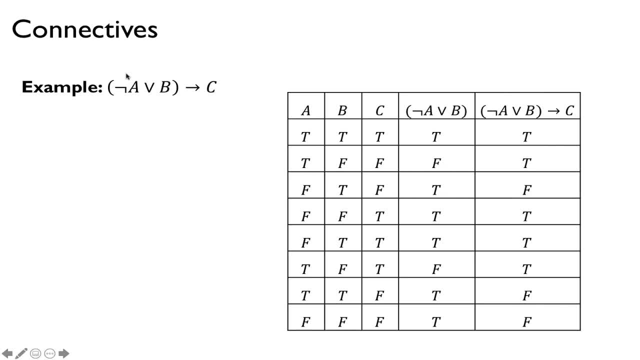 And this is the corresponding true table. So one way of doing this is to do one thing at a time, to do the A part first, the antecedent first, the premise of this, the conditional sometimes this is called. So you do this first. 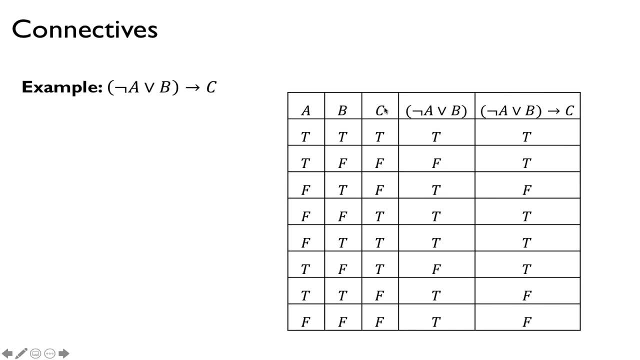 make a column out of it and then combine that with C and then relate this column to this with the conditional. So I'll let you guys check this true table And the key here is that once you have this, then it's easy to do the next part. 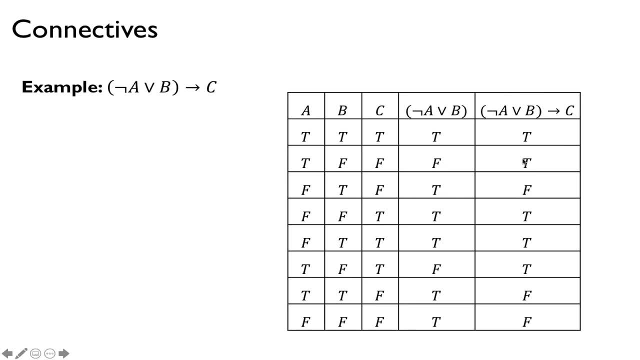 which is that, for example, let's do one of these. Why is this true? Well, if this is false, then it doesn't matter what C is, This will definitely be true. And then, as an example, if this is true and C is false, 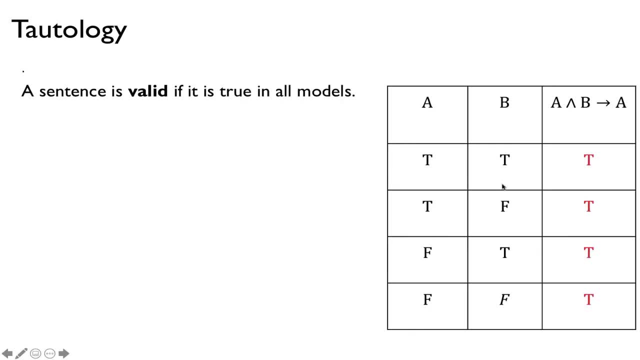 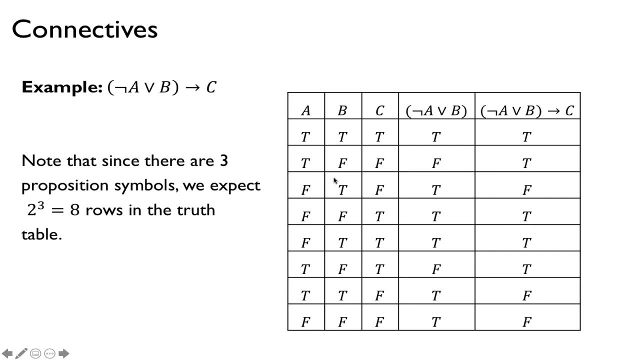 then that conditional will give you a false value. But go ahead and check the rest of that And notice that we have three symbols: A, B, C. So that means we expect eight rows in the true table, two to the third power. 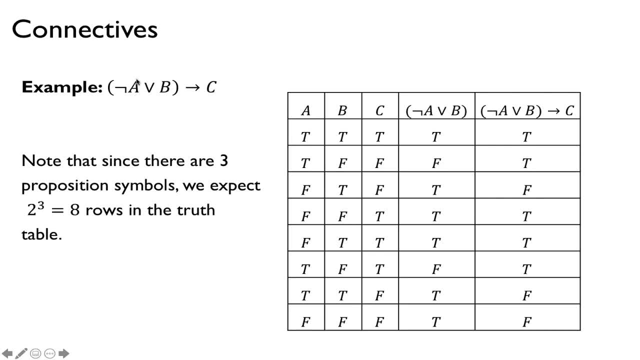 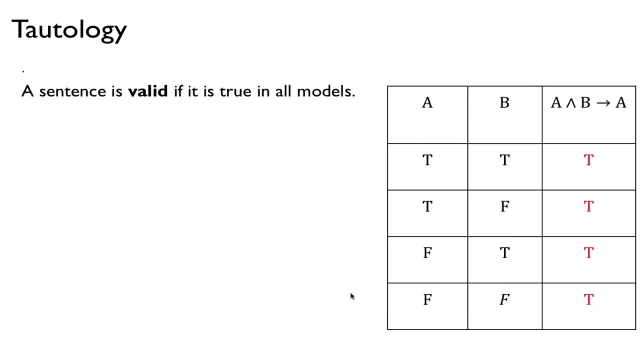 because every proposition symbol has two values. So two times two times two is eight possible combinations. Okay, So we say that a sentence is valid if it is true in all models, in all assignments. This is so. for example, A and B implies A. 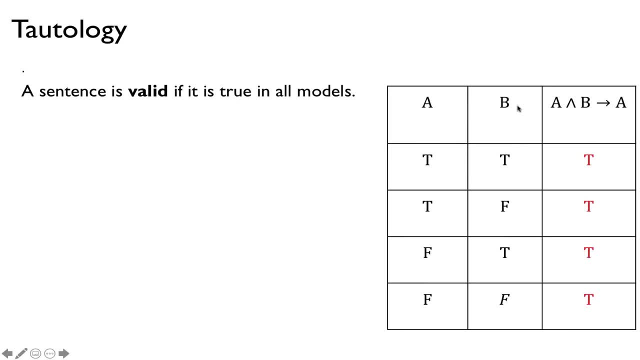 If you do this out, you get true everywhere. So that is true. So a model again, a model is just an assignment of true, an assignment of true or false to each of the propositional symbol, And so in each of these models, 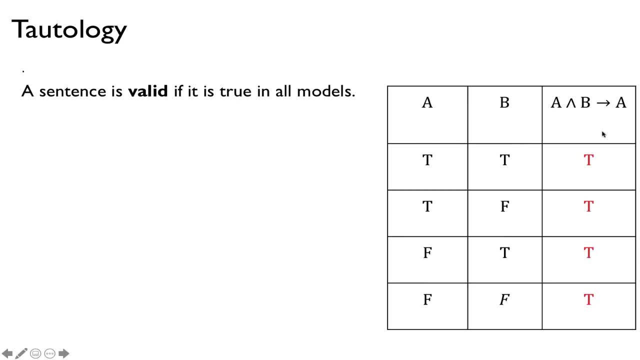 right. the answer is always true, So we say that this sentence is valid. It's always true, regardless of what assignment you make. Another example: is P or not P? This is always true. Whatever P is, either P is true or not. P is true. 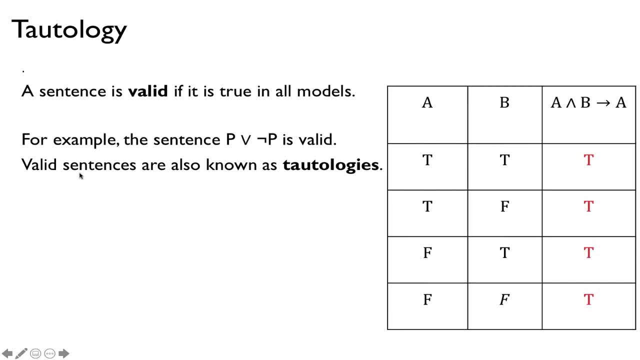 And so these are also known as the tautologies, And so valid sentences, tautologies, they're the same. So the determinant of a sentence is a tautology Or valid. we can use the true table If you use true table. 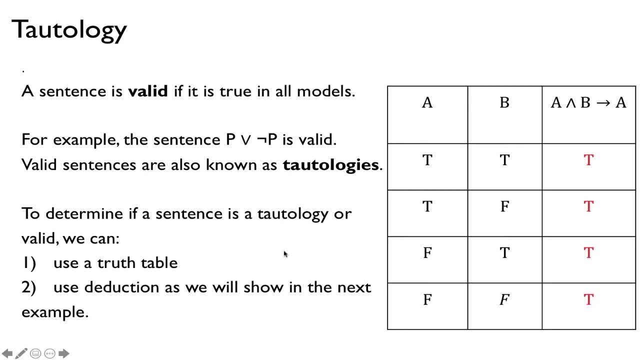 you get R true, then you know that the whole the true table is. you know that the sentence is true. So valid sentence is a tautology, And another way of doing this is to use deductions. So we're going to show that next. 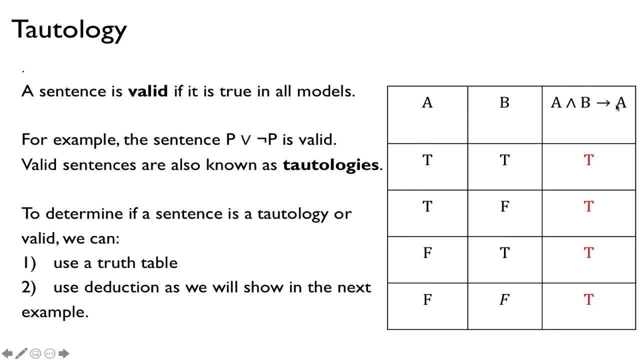 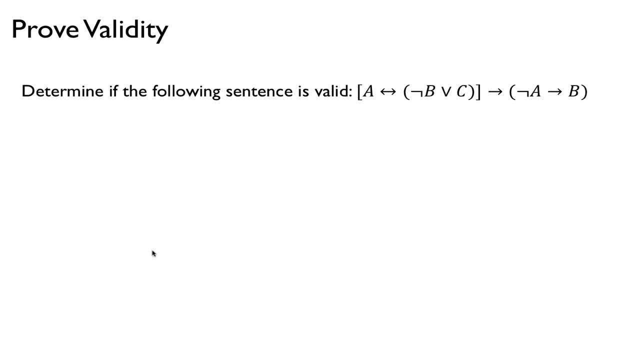 How do I use deductions to kind of reason? how do I know, use the definition of these operations and deduce that something is always true? So, for example, I want to prove that this sentence is valid. In other words, regardless of what A, B, C values are. 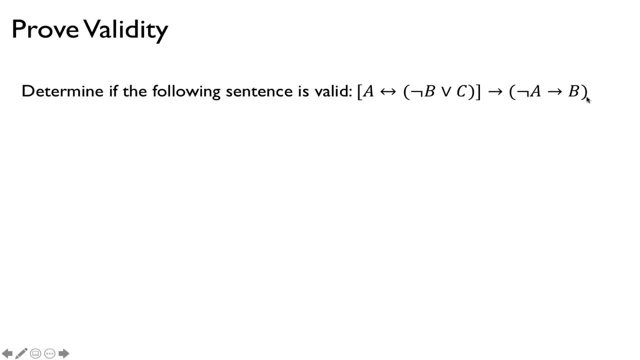 this whole thing will always be true. I'm missing actually. no, I'm fine. Okay, so here we go. So the way we do is that we're going to. we want to prove that this thing is always true, So we're going to use something called. 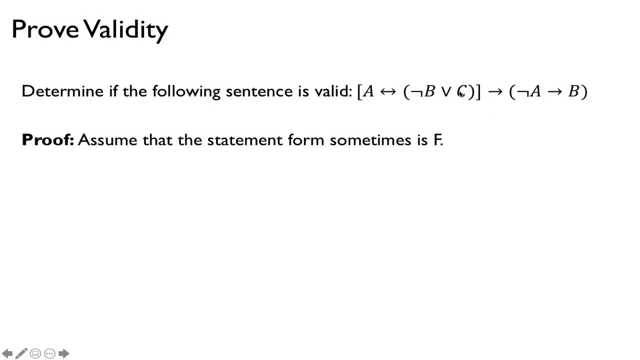 proof by contradiction And assume that there is some assignment of A, B and C that makes this false And see if we can get some kind of contradiction, And so so let's assume that for a second that this statement is false. 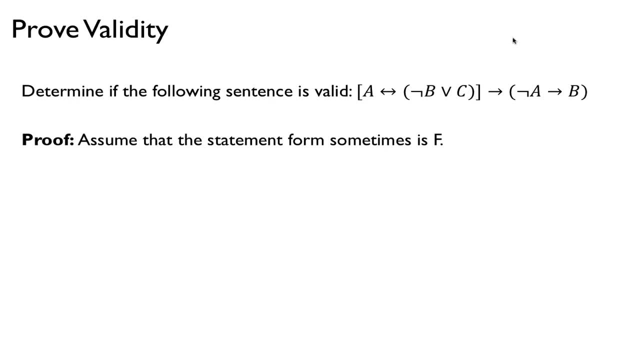 It's sometimes false, In other words, false for some value of A, B or C. Well, if this is false, that means that here's a conditional. Look at the outermost conditional here, the outermost operation, which is this one. 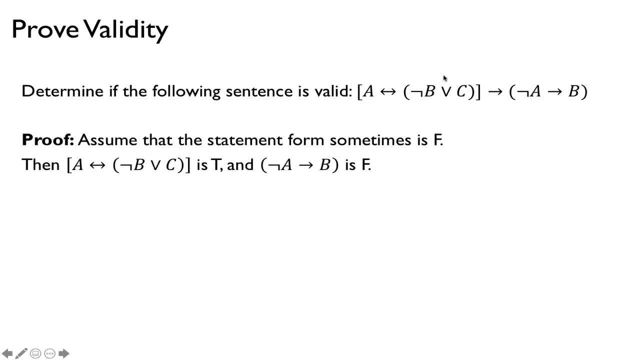 And say that if this is false, that means that this has to be true and this has to be false. So that's what this is. That means that the first, the first part of the conditional has to be true. the second is false. 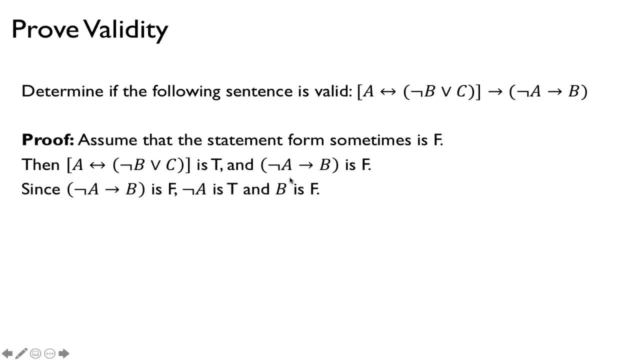 And then going off to looking at this, if this is false. and the next is that: if this is false, let's see what can we get from this. If this is false, that means that this must be true and this must be false. 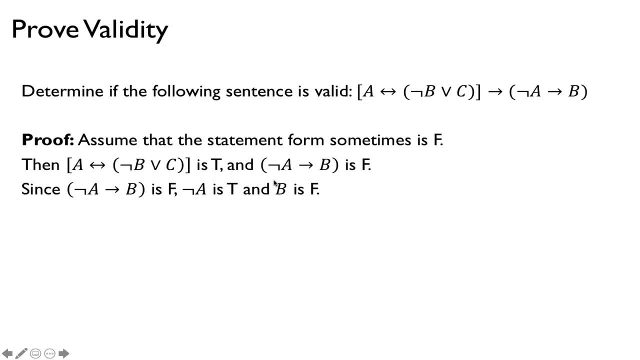 So not A has to be true and B has to be false. So now, based on our deduction, we know that B has to be false, be false. But if not A is true, that means A has to be false. and then, since B is false, 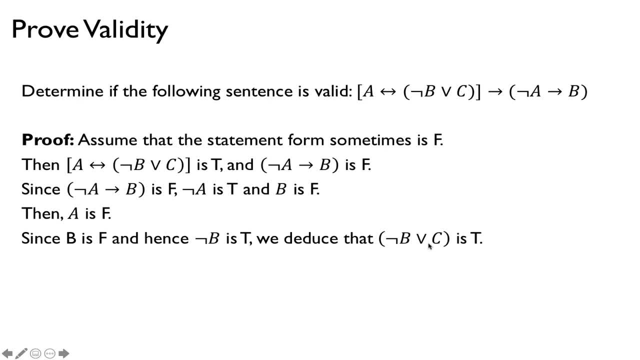 not B is true. we can also deduce that If not B is true, then true, or anything is always true, because this is an or so. if one of them is true, then the whole thing is true, But if A is false- we saw that earlier and this is true- we just proved that then- that. 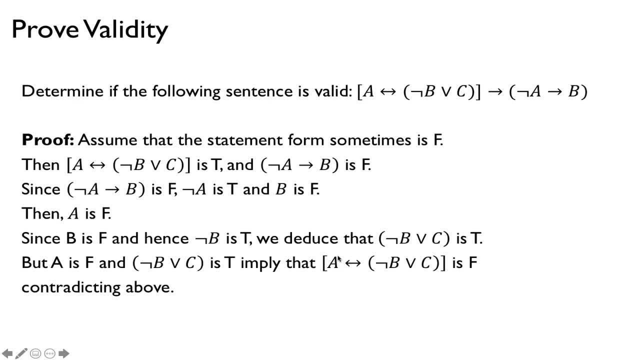 means that if this is true and this is, if this is false and this is true, then these are not equivalent. so this biconditional must be false. but that's a contradiction because we assume earlier that we proved earlier that this is supposed to be true. 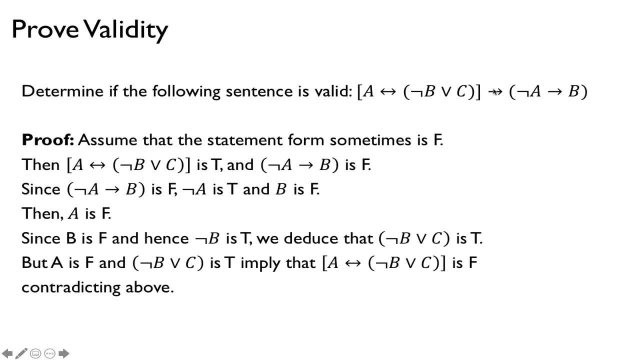 So that's a contradiction. that means that assuming that the assumption that we make, that this is this could be false or sometimes false, is wrong. therefore it must always be true. So make sure you understand that that logic. It's um. 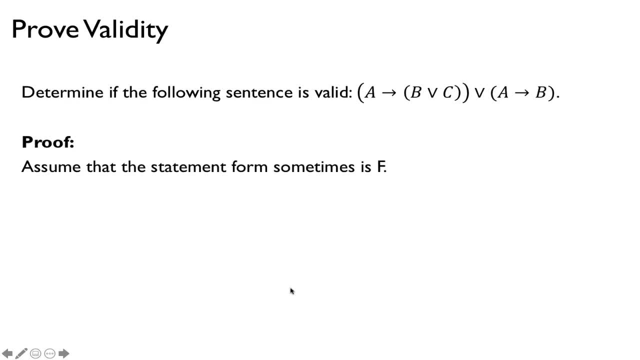 This is uh, proved by contradiction there. We'll get back to that a little later. um, Okay, so let's talk about how, about? how? about this one? let's try to prove that this is always true. Well, again same idea. we're gonna assume the whole thing is um is uh. 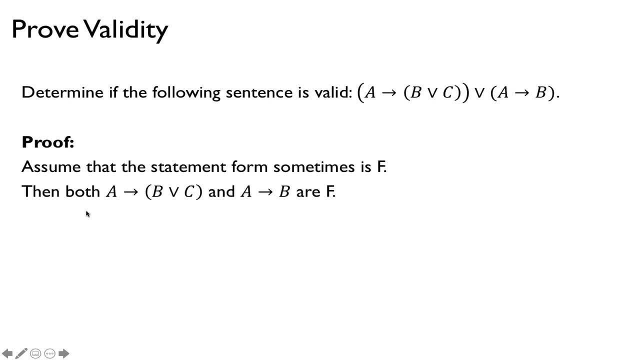 is false for some value and see if we get a contradiction, So uh it. so that means we're gonna. here's the outermost uh operation, the or. so if this is uh false, that means 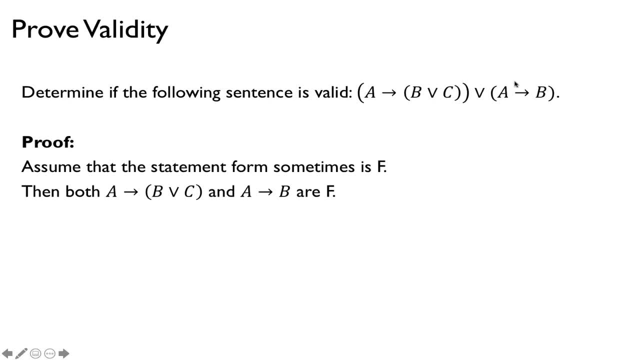 that this is false and this is false. That's how you get uh to be false. if you have an or so, that means the first part and and the second part are both false. Um, and on the right side, A uh implied or A by. 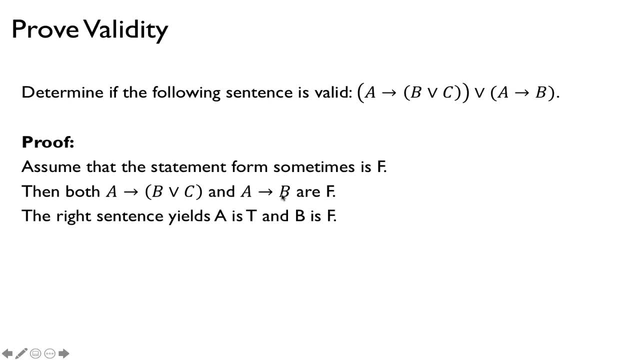 uh, condition of B. if this is false, A must be true and B is false, Uh, and then if A is? uh, if A is true, and um, let's see if A. yeah, if A is true here, uh, well, we. 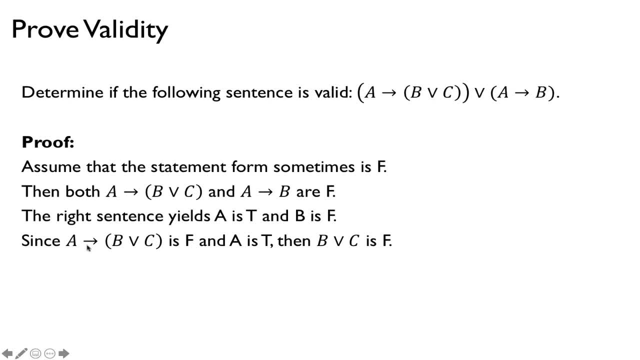 know that this thing is false from from before. If this whole thing is false and A is true, that means B or C must be false. So that's what that that says. Right again, this we know this whole thing is is false. but 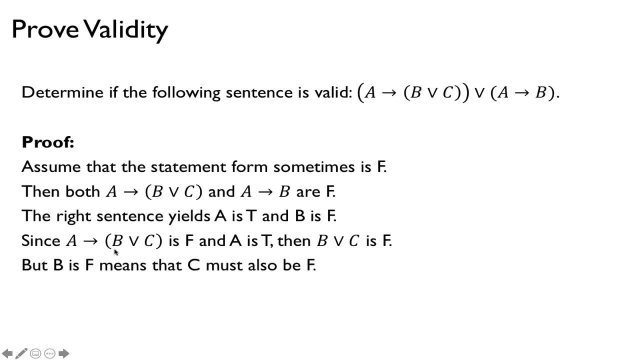 we know A is true, therefore this must be false. But we also already know that B is false, so that means that C must also be false for this to be false. So notice, right, every everything here we deduce by using the definition of these uh connectives. And so but notice. 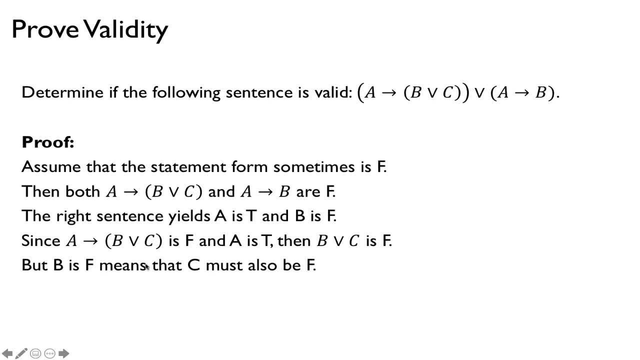 that we don't have any contradiction. We found that A is true, B is false and uh, B is false And C is false. So we actually found a model. again, this is an assignment: A is true B. 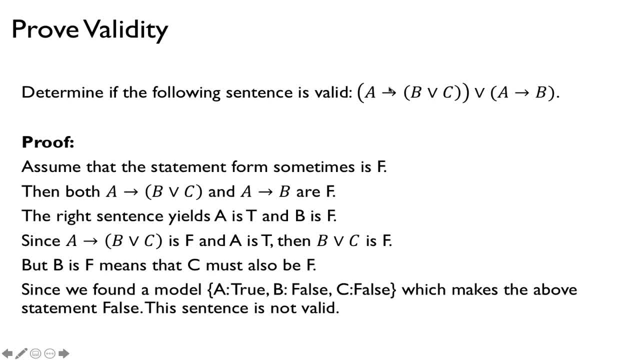 is false. C is false, And if you make that assignment, then this thing is false, And so it is possible that this is false. So that means that this is not valid, because valid means it has to be always be true The fact that we found one assignment or one model. 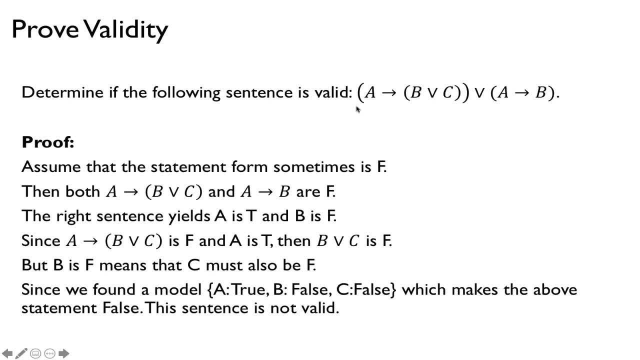 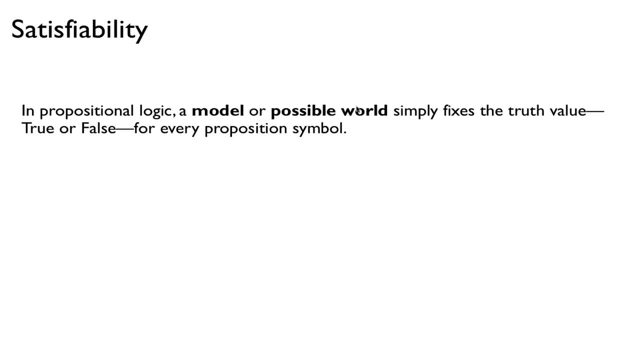 that makes this uh false means that it's not a tautology. the sentence is not valid. Okay, satisfiability, Uh. so in propositional logic, again, this is the uh, our next, our knowledge representation. language is the way we represent knowledge So far, using symbols. 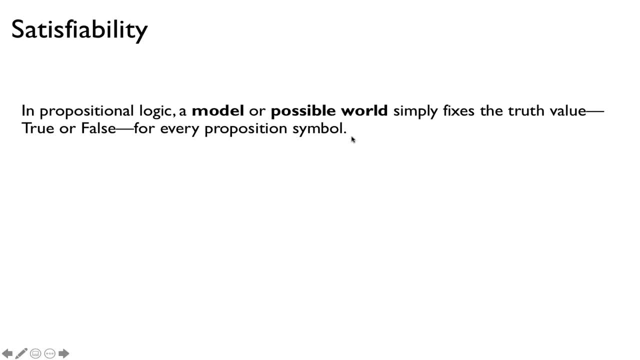 and these connectives to create these senses. So again, we kind of alluded to this earlier. but a model or a possible word simply fixes the truth, value, true or false to every proposition. symbol Just fix, assign a certain true or false to all the variables. that's a model. 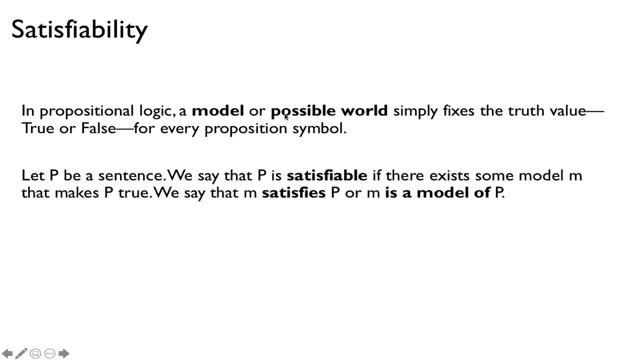 or a possible word, a possible state of a sentence. So if P is a sentence, we say that P is satisfiable. if there exists some model M that makes P true, If there's a way to make to assign all the variables in the, all the symbols in the proposition P to make. 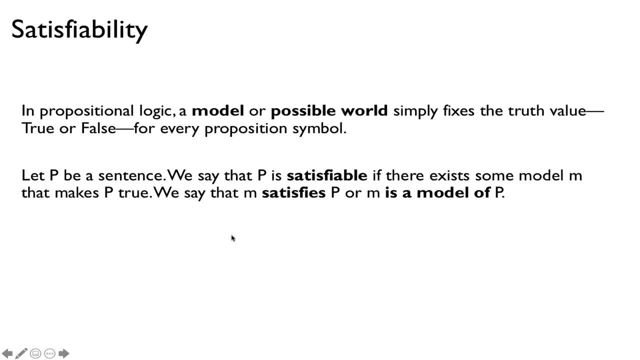 P true, then we say that P is satisfiable. We say that this model, this assignment, M satisfy P, or we say that M is a model of P. Now you have a. that's one sentence. what if you have a bunch of sentences, a set of? 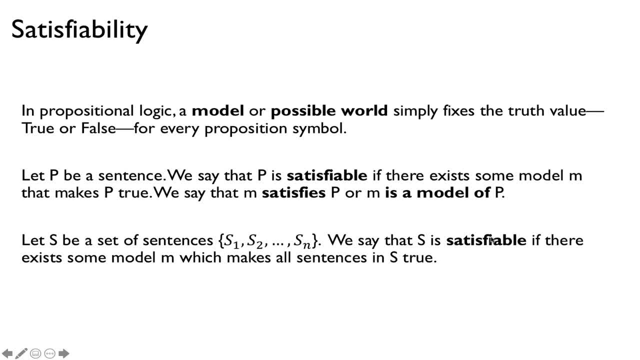 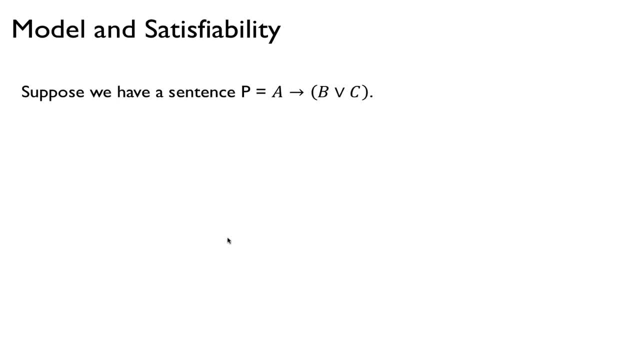 sentences S1 to SN, we say that S is satisfiable if there exists some model that makes all of them true at the same time. So, for example, here's P, one possible model: if A is true, B is false and C is true, that'll make P be true. you can check that out. So this model. 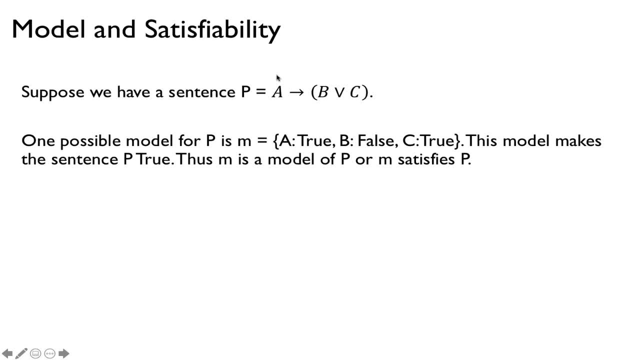 makes the sentence P is true. so we know that P is satisfiable and in fact this model satisfies P. I know this. we have three symbols, so we have two to the third, which is eight possible models. So we saw earlier that we have two tables. we have eight rows because there's 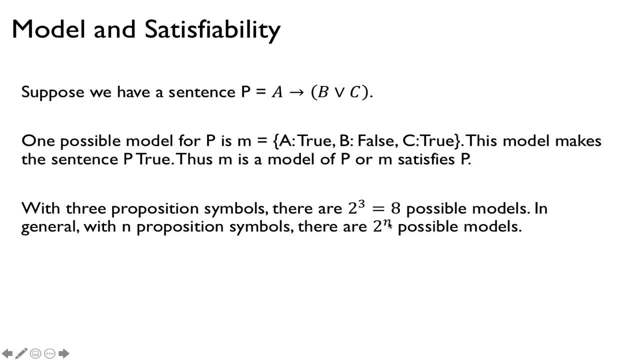 eight possible models. In general we have N symbols. then you have two to the N possible models. Noting this is an exponential function. That's why truth table- when you try to create truth table, it could take a long time. it's very expensive to do truth table because this: 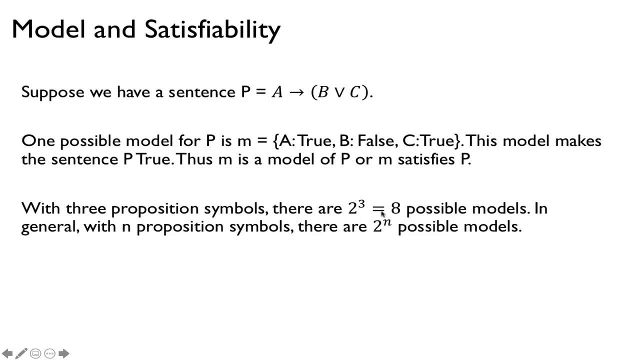 is exponential. So if N is- A are like a hundred, This is huge. So a truth table is simple, but it can be very computationally expensive. We're going to denote MP, to denote the set of all models of P, all the assignment. 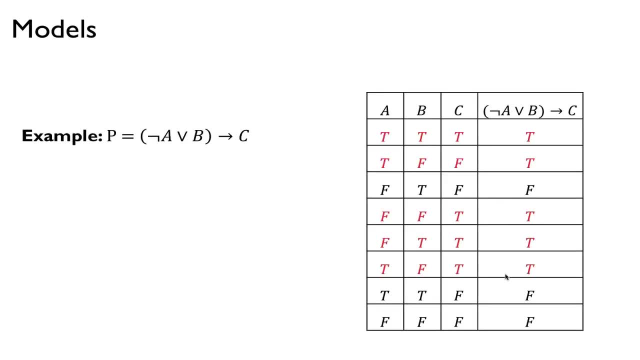 that make P true is M of P. So, for example, here's the truth table for P and notice what is M of P. M of P is basically all the assignments or all the models. This is one model, this is another model. There's five models in red. that makes P be true, and so that's what M. 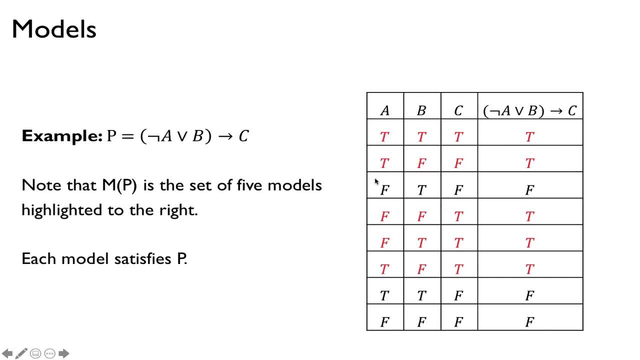 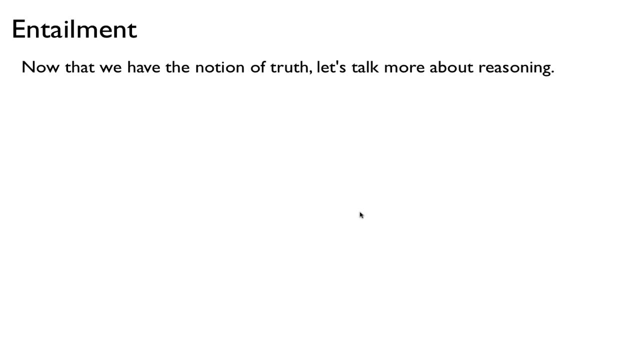 of P is M of P is these five models that make P true. Each model satisfies P. So that's what MP is. It's just the set of all these models, five of these models. Okay, entailment. Let's talk about what that means. So now we're going to talk about the idea of truth. We 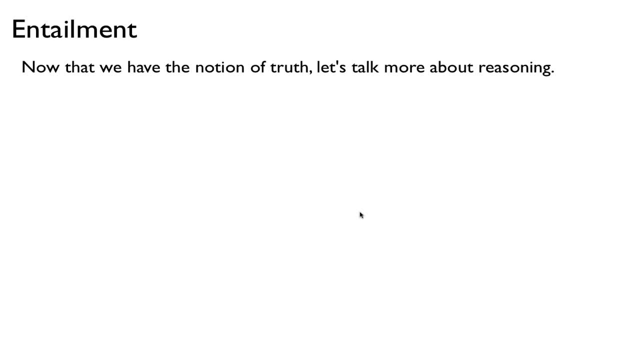 just discussed the idea of truth. Now let's just talk about how to reveal the truth. So let's just talk about how to reveal the truth. So let's just talk about how to reveal the reason with those truths. So this involves something called logical entailment. So the 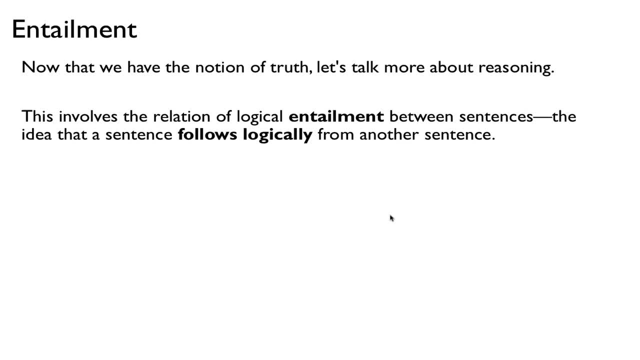 idea here is that we have sentences and we want to kind of figure out whether there's a relationship, whether one sentence follows largely from another. So logical entailment means that can we show that one sentence follows largely from another sentence. So for example, more formally, if P and Q are sentences, then we say that sentence P and. 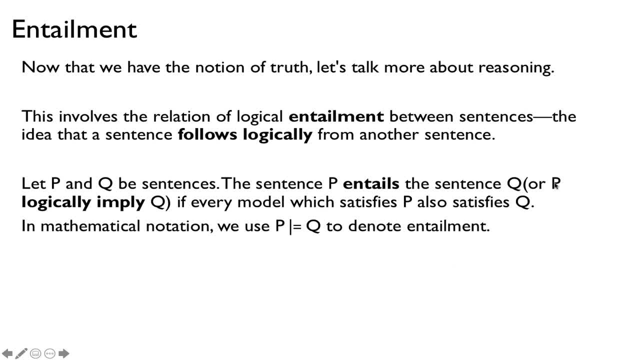 Q entails the sentence Q, Or another way of saying that is that we say that P largely imply Q, If every model which satisfies P also satisfies Q, And the notation we use for this is this notation. This is the vertical bar and inequality. This is used to show entailment. 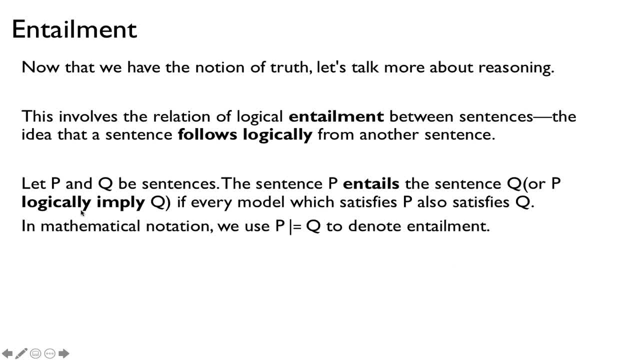 or largely imply, or logical implication, however you want to say it. There's a lot of ways for us to say this. This is logically entail In general, you have a set of sentences, S, S1 to SN. Then we say that S largely imply. 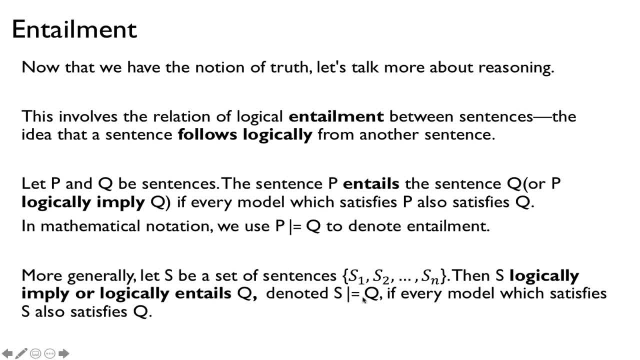 or largely entails Q. We denote, use the same symbol Again. before P was one sentence, but now you can have a bunch of sentences. So now it's the same definition. It means that every model that satisfies all of S must also satisfy Q. So again a set of sentences, largely 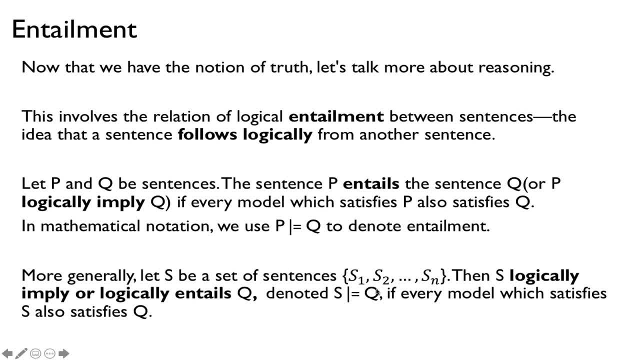 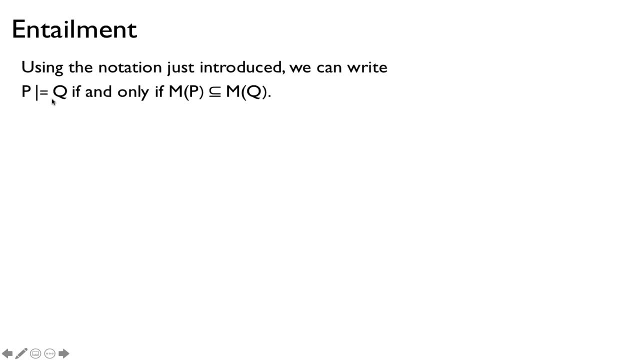 imply or largely entail a sentence Q If every model that satisfies all of the sentences also satisfies Q. So this is the generalization of this definition. So, using the notation earlier with the models, we can write that P entails Q if, and only if, all the models of P is a subset of the models of Q, In other words, any model that 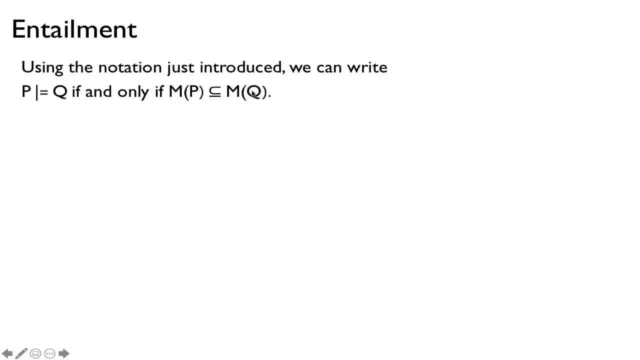 makes P true also makes Q true, And so these two statements are equivalent. If P entails Q, then the models of P must be a subset of the models of Q. Another thing about this is that P is a stronger assertion than Q. That's a typo here. 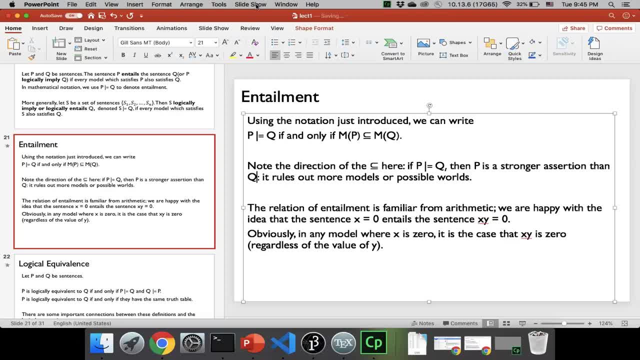 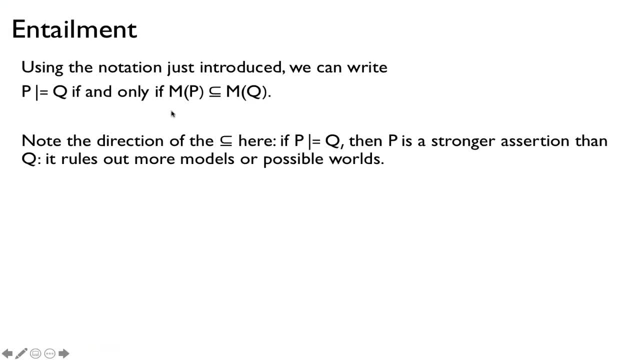 What is that? Let me explain that. So the left side of this: this is a stronger assertion than Q because notice that this subset is, this is a subset of MQ. The reason why this is a stronger assertion is because it rules out more models of possible. 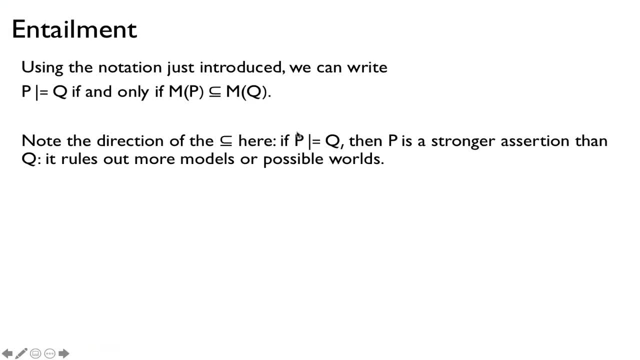 war, All right. If something is stronger assertion- you have more conditions, more constraints- then it rules out more possibilities. So, for example, if you're trying to come up with a characteristic of someone you want to date and you have a lot of conditions, a lot of you have a kind of a strong you. 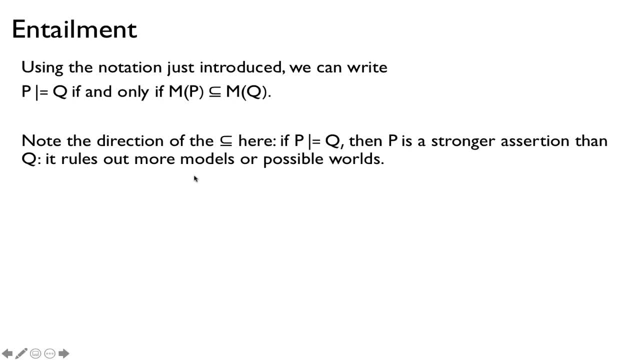 a strong constraint, then that means that you're going to have less people who might satisfy those conditions. So yeah, in this case, P is a stronger assertion. That's why this is a subset: because you have a stronger assertion, you have less models that satisfies. 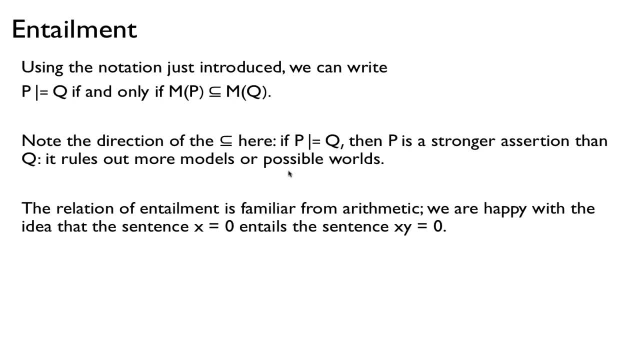 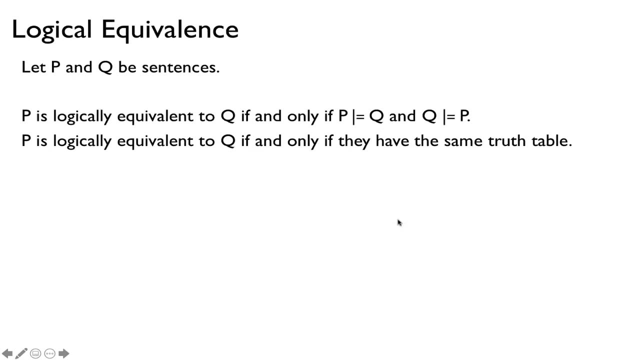 it. So, as an example of entailment, if you have the X is 0,, then that largely implies or largely entail, X times Y is 0. If X is 0, the product of X times Y, regardless of the value of Y, is also 0.. To solve for logical equivalence, you have P and Q as sentences. 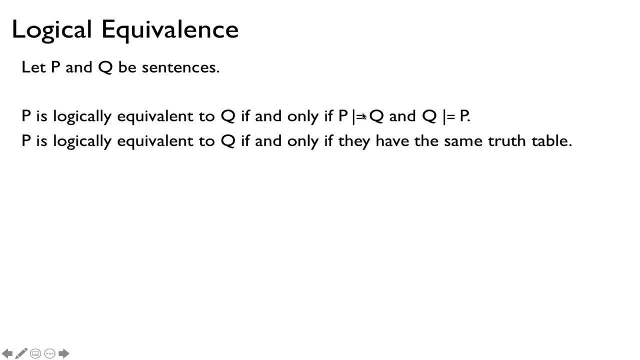 P is largely equivalent to Q if, and only if, P entail Q and Q entail P. Another way of saying that is that P is largely equivalent to Q if, and only if, they have the same truth table. So there is some important connection between these definitions and logical connectives. 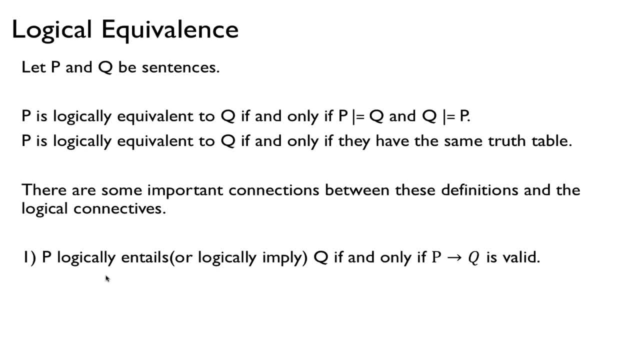 And so I'll say right here, and some of these will be done in the homework, but I'll just say that, And also, this is really simple: If you look at the definition, this is followed from the definition, but P largely entails or largely imply Q if and only if, P conditional. 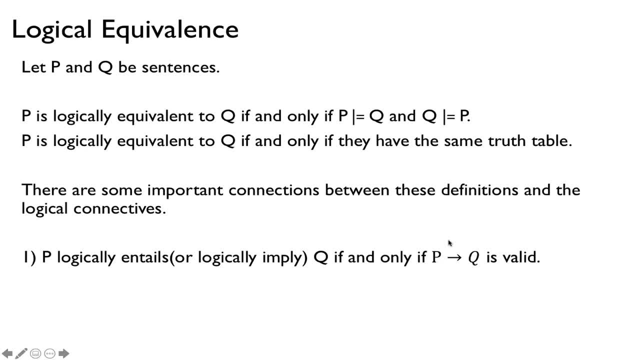 Q is valid. So if this is always true, if P implies Q is always true, that means that P entails Q And, conversely, if P entails Q, then that means that this connective is always valid- is always true, So that this connection between the connectives conditional and 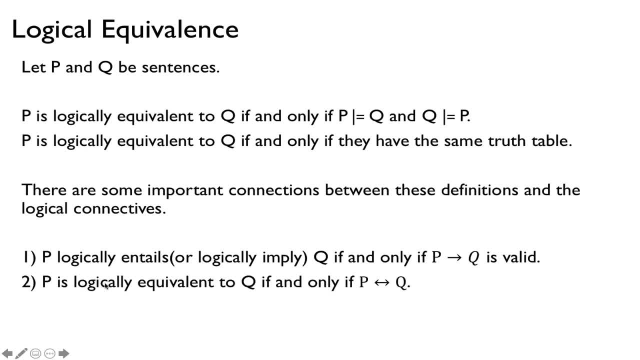 largely entails. In the same way, largely equivalent is related to the biconditional upper connective. So these are similar in that way. There are equivalent in that way. Okay, So here's another example. Here's P, If P entails Q. if P is larger, equivalent. 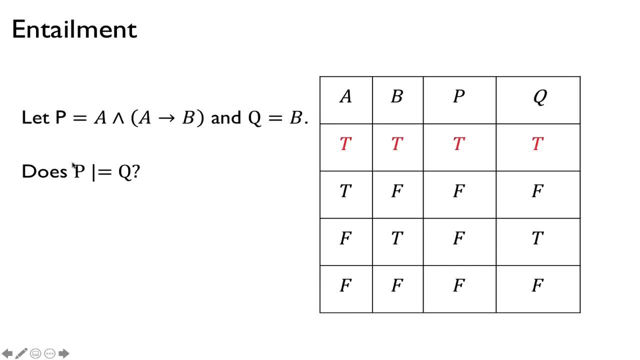 here's Q and the question here is: does P entail Q? In other words, if P is true, is Q true? Well, look at the true table and see that. look at all the models. there's four models, four assignments. 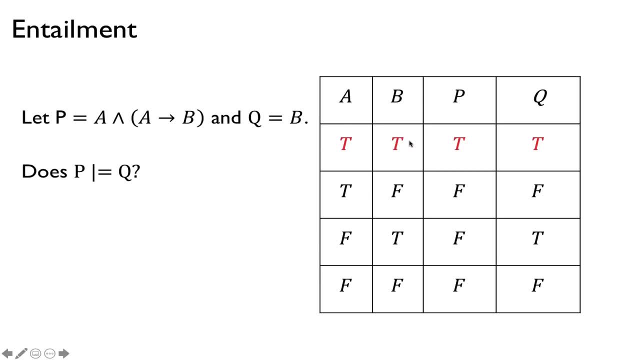 here and notice that the assignments, the model, this model that makes P true, also make Q true, Then it makes P false, then we don't care. So we don't look at these three lines, We only care. entailment means that: 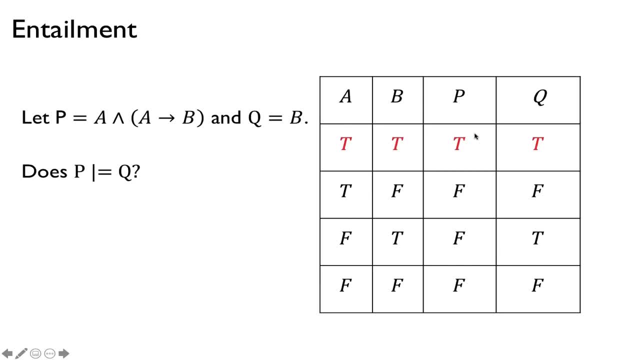 if P is true, Q must be true, and there's only one rule that satisfies that condition: that the assumption that P is true and Q is also true in that case. So P does entail Q, So this statement does entail this statement. So this statement largely implies this statement. So that's another way of thinking about that. 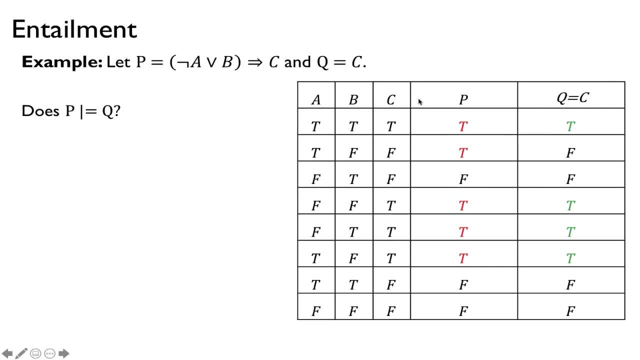 How about this one? Let's say P, is this one right here? and Q is C. Does P largely imply Q? Well, we look at this and say, well, actually this line right here, P is true, but Q is false. So that means: 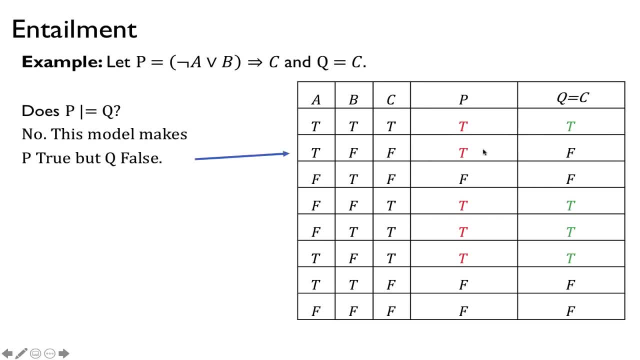 that the answer is no. This model makes P true, but makes Q false. so P doesn't entail Q or P doesn't imply Q. How about Q? Does Q entail P? Does Q largely imply P? Yes, because every time Q is true, P is true. Here's another model. 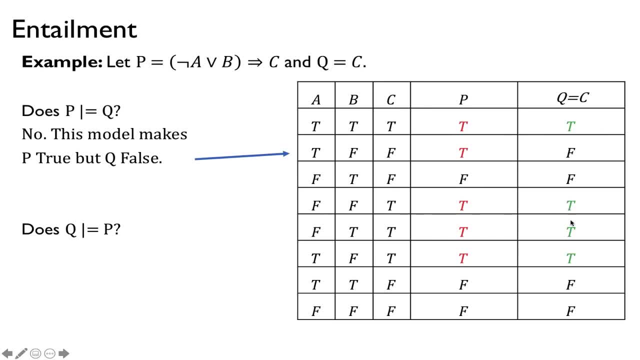 This model, right here, Q is true, P is also true. So every time Q is true, in other words, the set of MQ, four, these four things, is a subset of MP, these five, five models. so notice that subset definition. so this is the answer here is yes, every model which makes Q. 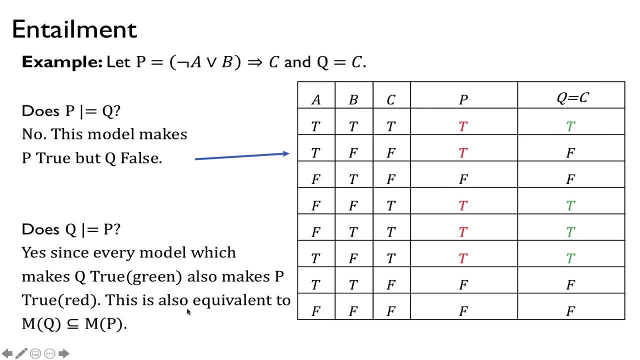 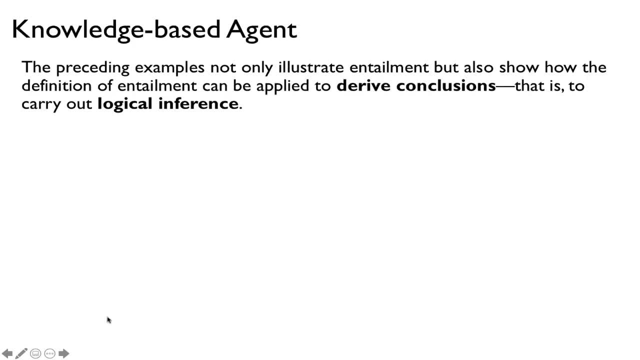 true the green also makes P true the red also notice this. the set of models of Q is a subset of the set of models of P. okay, so knowledge base agent. in the previous example we use entailment to. actually we use entailment to to derive conclusions. so this is kind of a nice that we can use truth table and 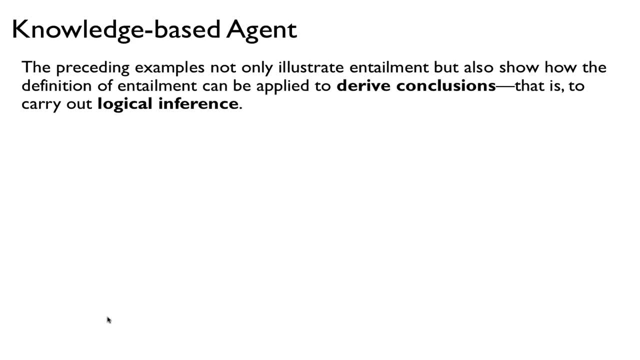 entailment to, to make logical inference, to take truth and also to derive new truth. so that's, this is nice, that we can actually reason with them with the entailment and truth table. so when you talk about knowledge base agent- an agent who has knowledge and who can apply that, 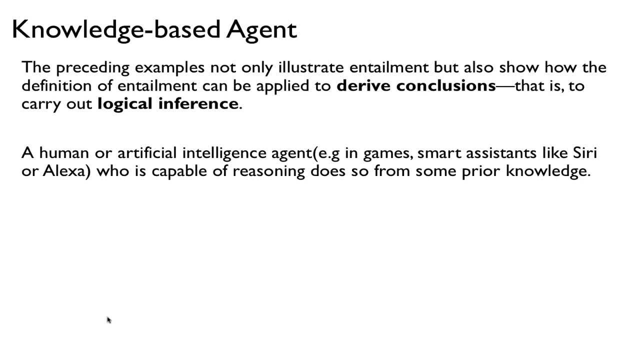 knowledge by deriving conclusion and making logical inference. for example, a human will be a knowledge base agent or an artificial intelligence agent, for example, in games. you play games in some of those AI players right can, can make decisions and can be very smart, or even something like Siri or Alexa smart. 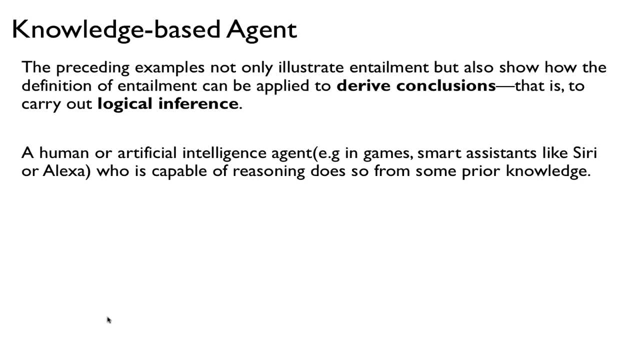 assistant like that. they, they have a certain knowledge base and they, they can actually deduce and make conclusions and an inference and and all these things have have. they have some kind of prior knowledge they have that they can work with. and so we say that a knowledge base- or KB for short, knowledge base- is basically a set. 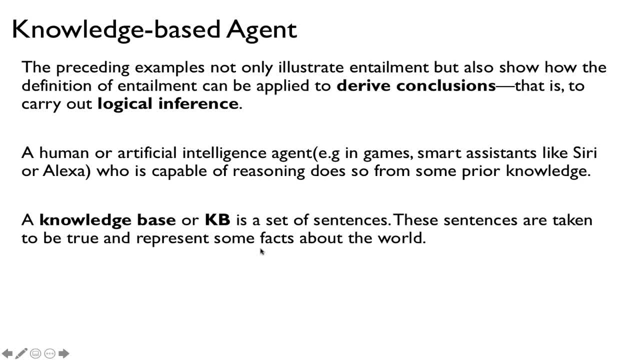 of senses, and these senses are taken to be true and represent some facts about the world. so this is basically a bunch of senses that we're going to assume to be true. so we call that the knowledge base. so, humans, we have knowledge base with that, we work with everything, we know, everything, we learn, and then even 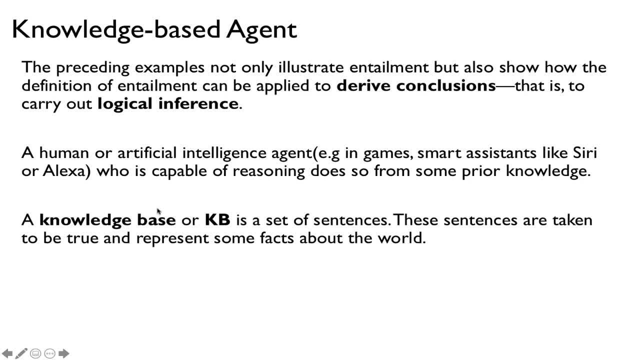 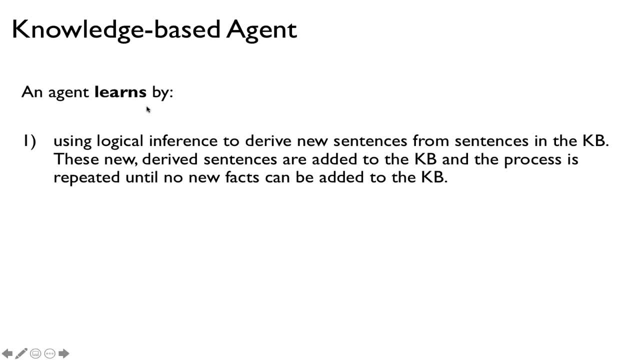 something like Alexa Siri. it has a certain knowledge base that it works with. so that way, when you are given knowledge base, the way that you're actually learned this is that it works with the sense that you've two senses, so an agent learns by. well, a couple ways is that we can use logical inference to derive new senses. 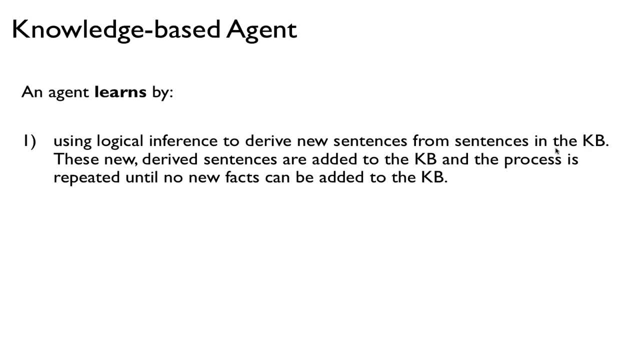 from senses in the KB. so I have a bunch of- not a fax- from the KB, the knowledge base. I can use deduction to produce new senses, conclusions or in fences, and then that's how I, one way I can learn and they can. I can take those new facts, those 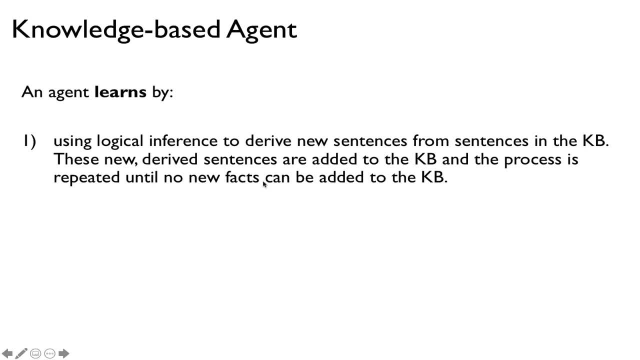 new, derive senses and add it to my knowledge base, conclusion, to your knowledge base, and then that's one way to learn. Another way to learn is: you just told the new facts. Maybe you program something, you add facts to Alexa or whatever, or maybe you have a robot. 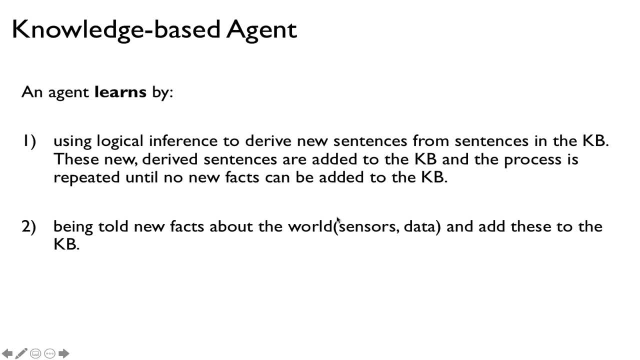 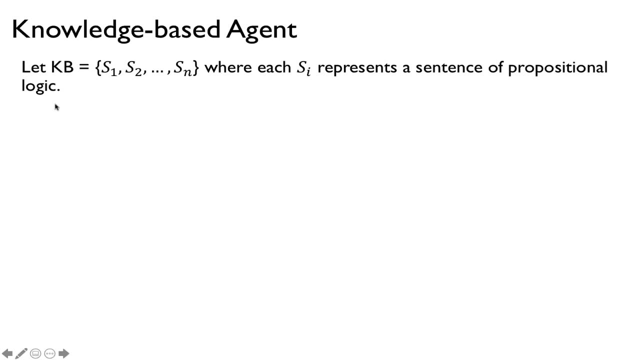 that has sensors or data that it's collecting. as it sends data around it, it's learning new facts about the world it's living in, so it can add these to the knowledge base. These are two ways that an agent can learn, And so KB, the knowledge base, is essentially a set of sentences- S1 to SN. each of these. 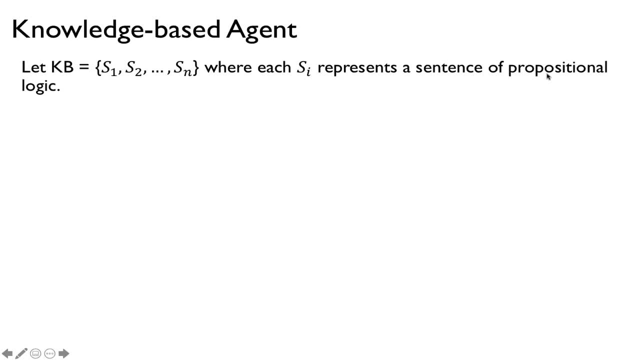 SI is a propositional sentence. so we assume that everything here is true and suppose that we have some propositional cue and we want to know whether our knowledge base entail cue. In other words, there's a knowledge base, Can we imply cue? 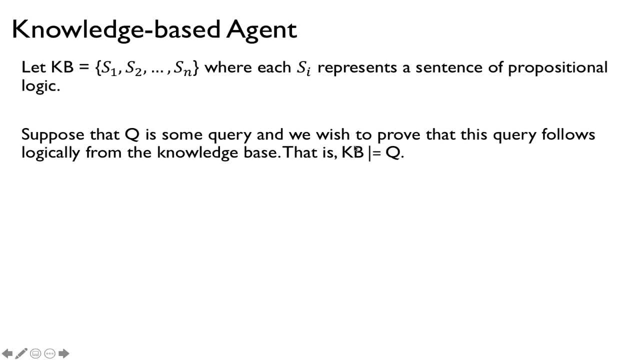 Can we derive this new sentence from our knowledge base? We can use the true table to carry out this logical reasoning. So this is nice, that even though the true table is pretty simple, it can also help us reason. That's what we want to get out here. 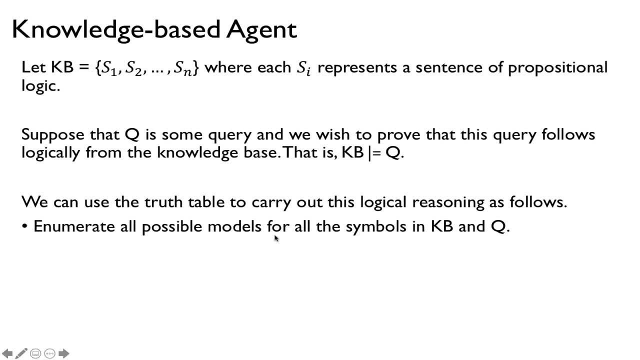 So one way to do this is that we enumerate all possible models for all the symbols in KB and cue. We just look at all possible assignments or models And we check that if every model, If it satisfies all the sentences in the KB, also satisfies cue. if that's true, then that 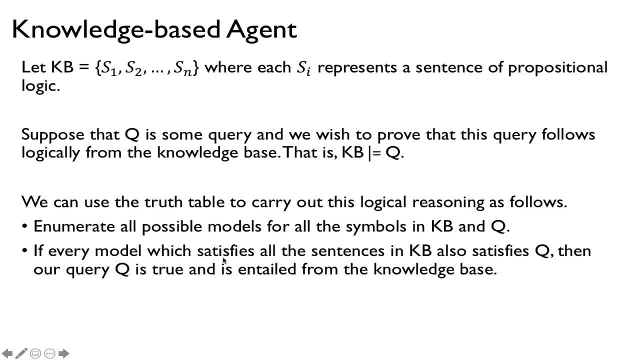 means that cue, that the knowledge base does entail cue. So this method of reasoning is also called model checking. In fact, we can actually write a program- and maybe in a future video we can use Python or something- to write a program that does model checking, that just use the true table. 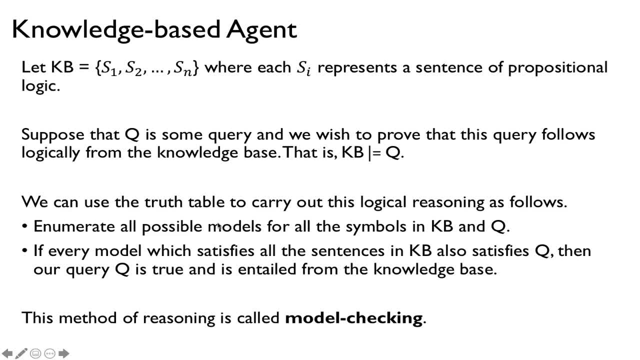 and just enumerate all possible models. Computers are very good at this: just enumerating all possible models And checking the definition of entailment. If the knowledge base is true, then check and see if this is true And then if this KB entail cue, then we have basically found a new fact. that is true, and 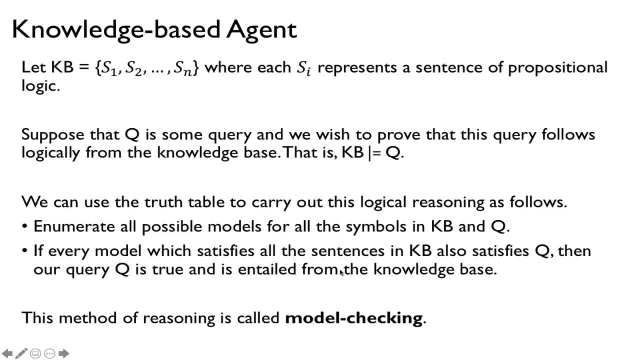 we can add it to our knowledge base. So this is one way to reason And model checking is just a brute force way of enumerating all possible models and just checking the definition of entailment. But if the definition is satisfied, then that means we have the definition of entailment. 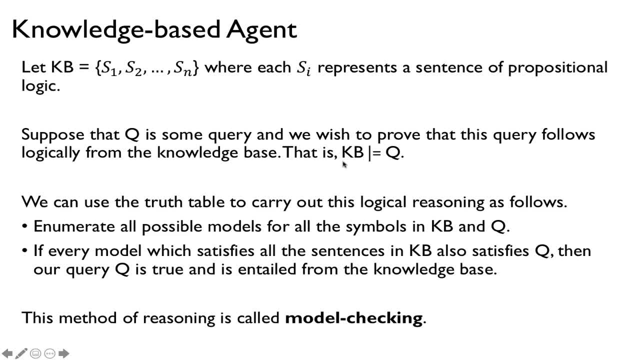 So that's the way to do it. We have reason and we have inferred that if KB is true, then cue is true. So this is called model checking And again, I think maybe in a future video, maybe next week, I can show you how to do. 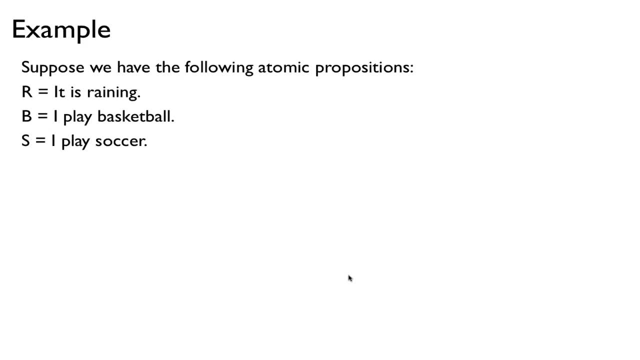 this with Python or something. Suppose that we have the following atomic proposition. Let's do an example here. So let's say R means it is raining, B is I play basketball and S is I play soccer. And suppose that we have a knowledge base, just a bunch of facts, and say that our knowledge 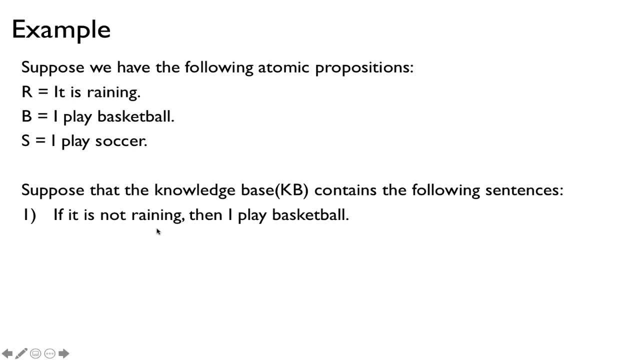 base contains the following sentences: So here's the first fact from our knowledge base. If it's not raining, then I play basketball. So maybe that's the fact about me. I play basketball or soccer, but I never play both on a given day. 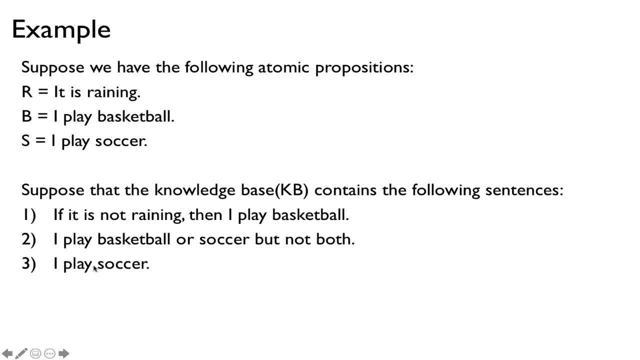 And maybe on a given day I play soccer. So if this is all the sentences in my knowledge base, can I deduce, can I make a deduction from this? Can I conclude, Can I derive or infer, Can I deduce? 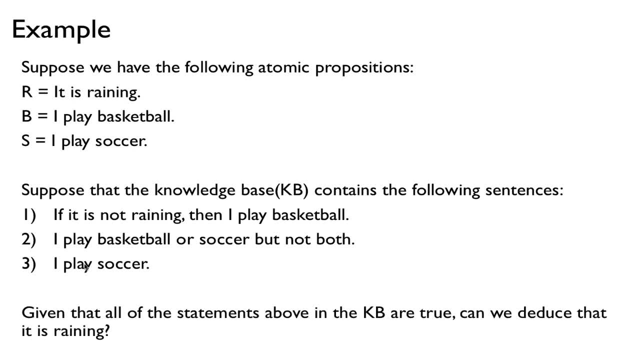 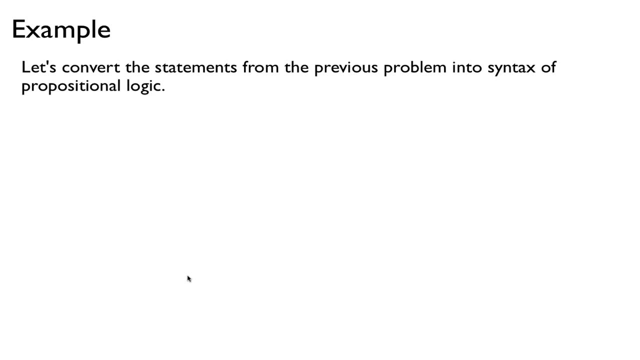 Can I conclude? Can I infer new sentences from my knowledge base? So, as an example, does my knowledge base does it entail or logically imply that it's raining? If these are my facts on a given day, does that mean that it's raining, for example? 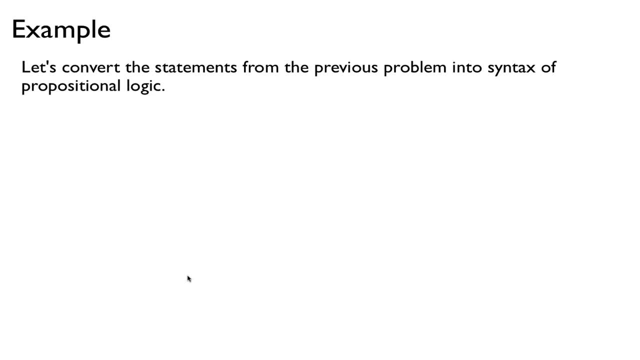 So let's convert the statement from the previous problem into a syntax of proposition logic. So the first one is: if it's not raining, then I play basketball. That says that not R implies B, So if it's not raining, I play basketball. 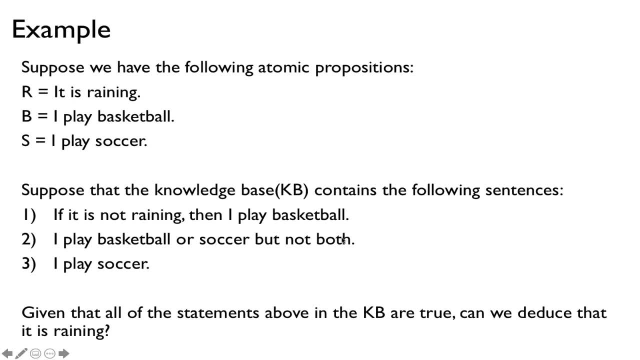 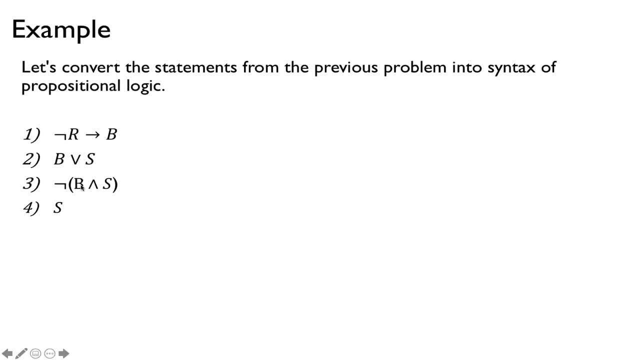 The next one is: I play basketball or soccer, but not both. Well, I can do that in two sentences. I'm going to say: I play basketball or soccer, but not both, Not both. So that's the second, just breaking this down into two sentences. 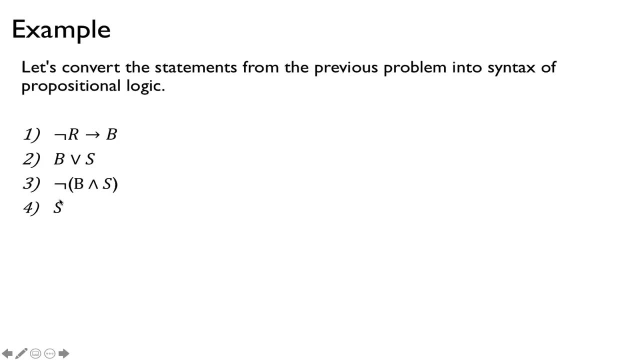 And then I play soccer means that S is true. So if I have, all this is my knowledge base. Again, knowledge base is basically just a set of sentences that are assumed to be true. Does this knowledge base entail, or logically imply, that it's raining? 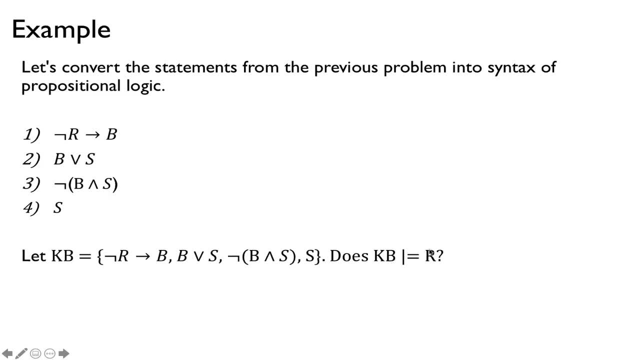 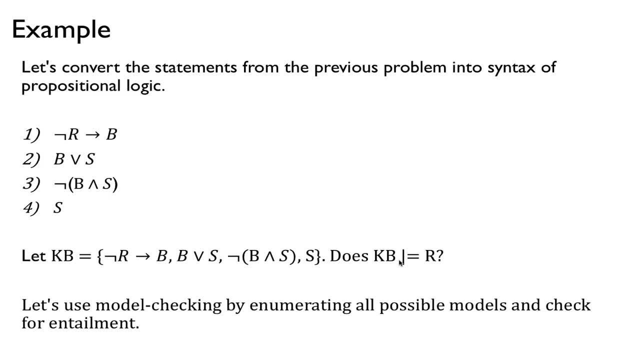 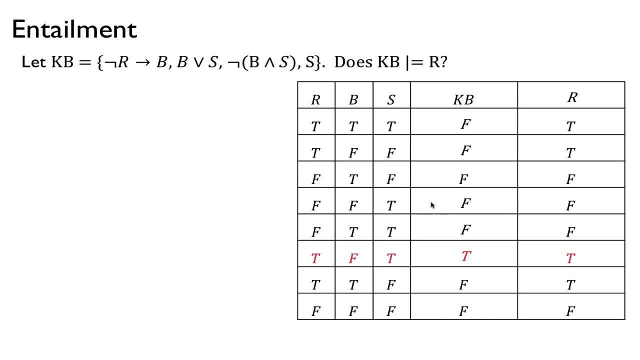 Does this knowledge base entail, or logically imply, that it's raining Right? So let's use model checking by enumerating all possible models using a truth table and check for entailment. So here's the truth table. Again, you can check the work here. 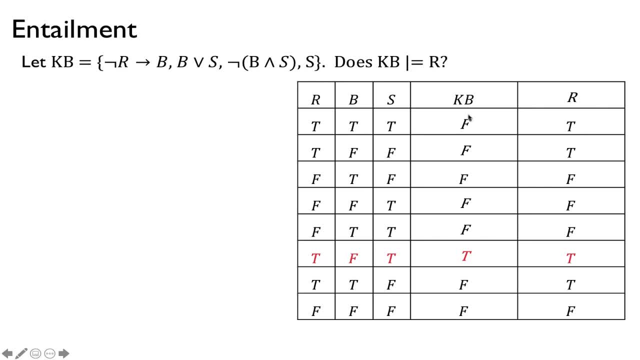 But notice that KB- this column represents the. basically, we have to check that for every model. We have to check to make sure that all of these are true, Because if one of them is false, then we get the false value here. So notice from here that there's only one model, this model right here in red, that makes the KB true, the knowledge base true, meaning that if R is T is true, B is F and then S is T, then it makes all of these statements true. 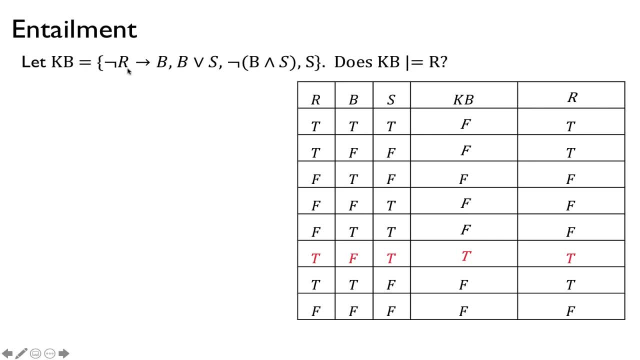 So you think of KB as an and right. Take each of these statements and then and them together. And so if I and them together, then the only way to get it to be true in this example is there's only one model here. 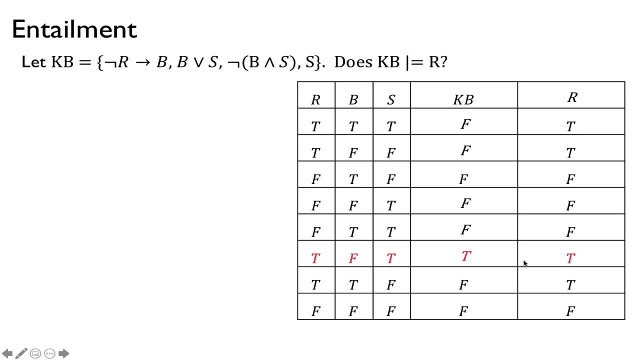 Well, in this model where it makes the KB true, it's R true. By the way, R I just copy and paste R same thing as this one. So there's only one model where it makes the KB true and that model also makes R true. so this does satisfy the definition of entailment. 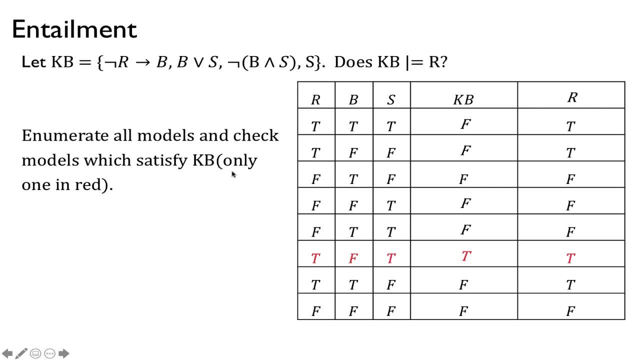 So we do. we enumerate all models and check that there's only turns out there's only one in red that satisfies KB. but it's enough, because that one also makes R true. so that means that we do have entailment, And so that does mean that, given this knowledge base of facts, I can conclude that it is raining. 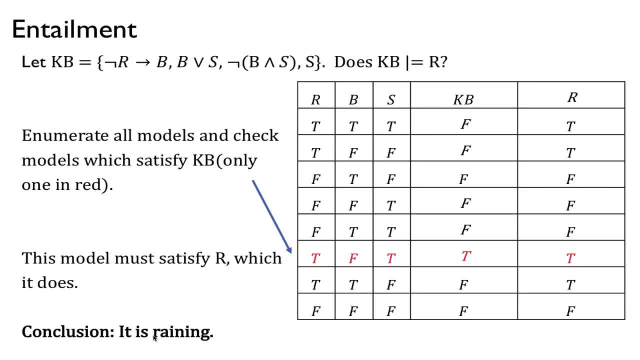 Yeah, so that's basically the end of this lecture. We talked about truth table, we talked about how to, we talked about sentences in propositional logic, how to combine them, how to, how to form them, and then we talked about how to use the truth table to reason, as in this example. 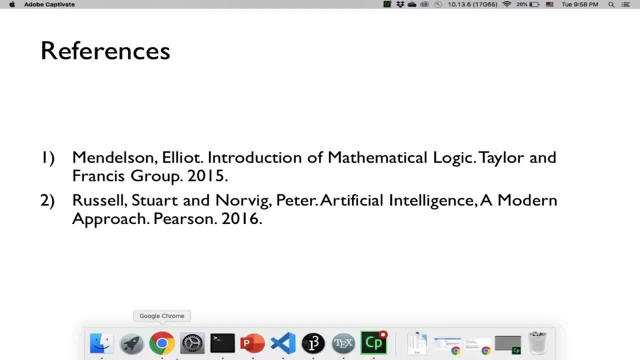 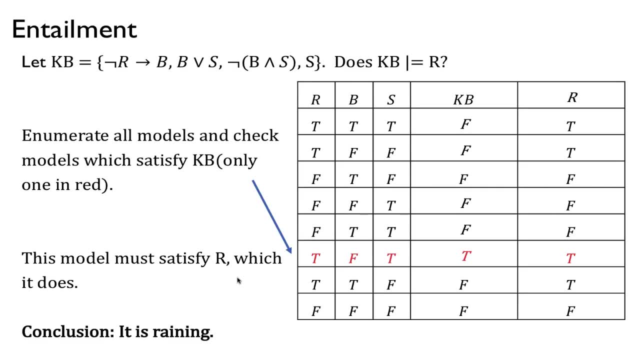 Yeah, so that's the first, so here's my resources. You're welcome to look these up, but okay, great, So I think I'll just end this lecture here. Okay, thanks for watching.